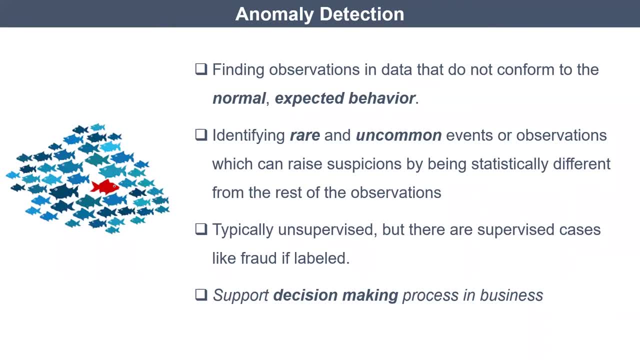 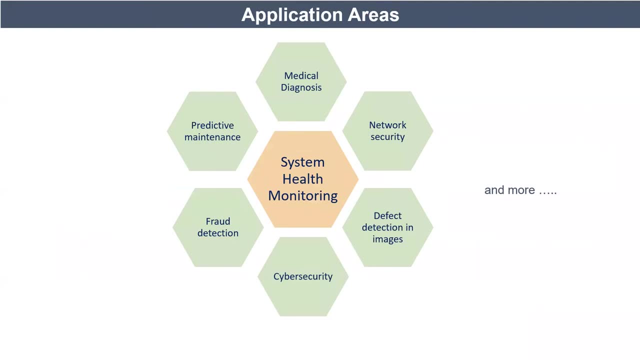 although I believe, especially if it is real-time decision-making, it's always good that it supports, but the people do not really only rely on automated decision-making. Some application areas are like system health monitoring. I have previously worked on like predictive maintenance and also again health monitoring. 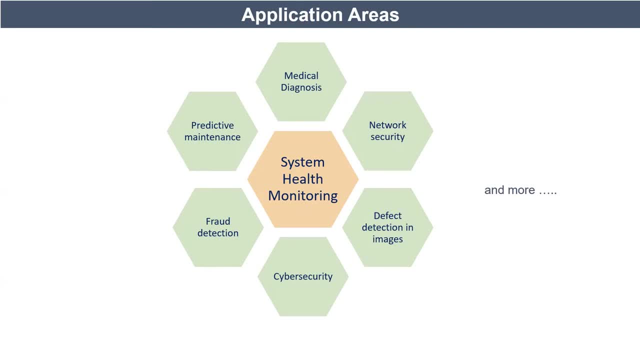 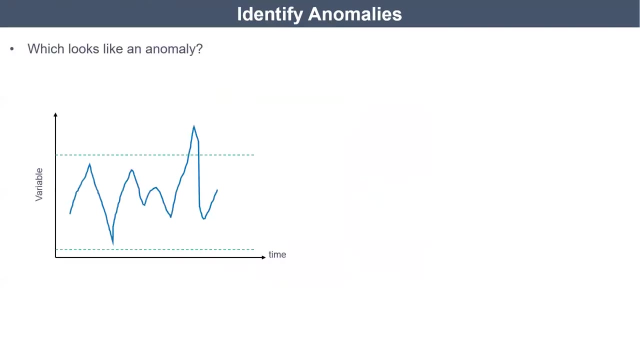 of flying systems. They are also used in medical diagnosis, network security, defect detection in images and manufacturing. basically cybersecurity and fraud detection and many more, obviously that I don't know Basically. I mean people are- I mean, in my experience are- used to looking at anomalies. 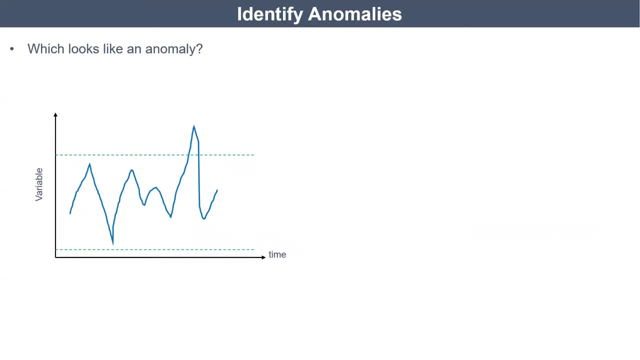 visually and just try to identify them like looking at this figure, This looks like an anomaly if it is really beyond the variance of the signal itself, I mean when it is univariate or bivariate. basically, it may be easy to identify those. 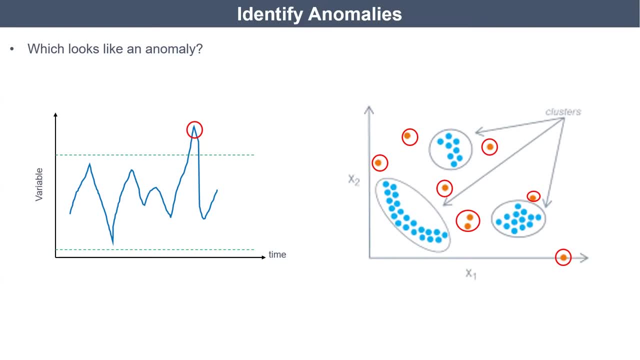 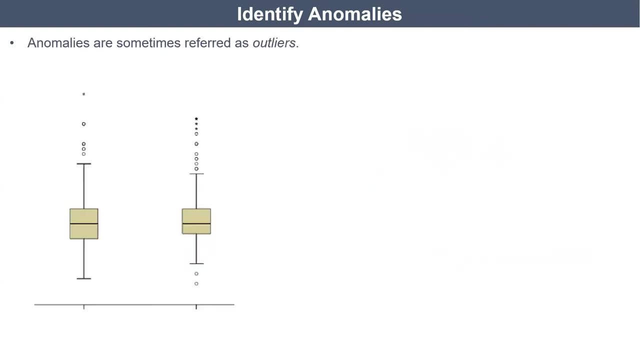 visually, but in multi-dimensions it's much more difficult. so we need some techniques to do that And they are also sometimes called as outliers and statistically also they are observed in box blocks and there's a method like this IQR range method, basically. 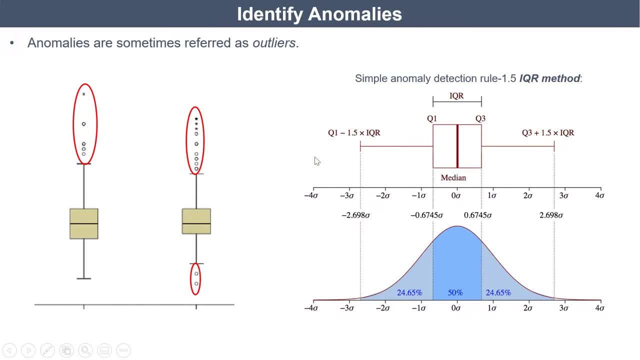 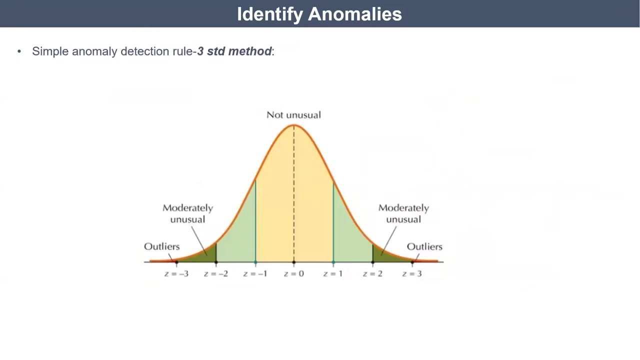 when the observations lie. So when the observations lie beyond this 1.5 interquartile range, then they are called as anomalies. Again, this is a simple approach. So beyond those points we call them abnormal. Similar to the interquartile range method there is also standard deviation method. So we say: 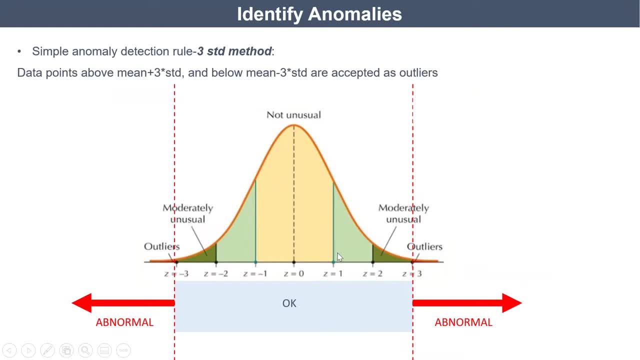 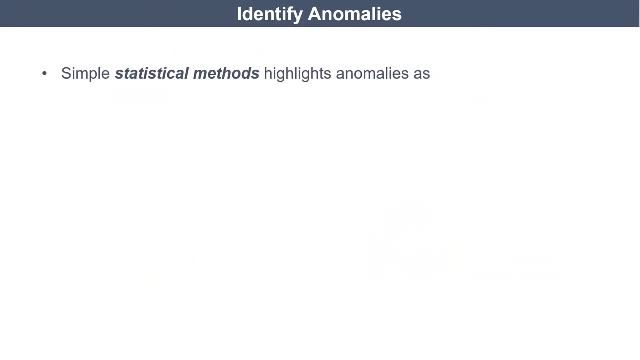 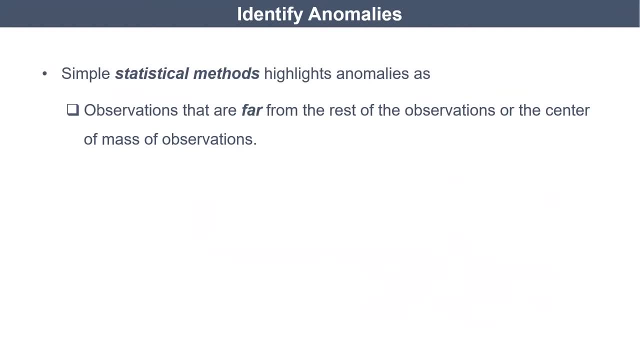 of the observations or a center of mass of observations. they are called outliers. that's easy to detect when we have one or two variables but or when we can visualize them in a histogram or scatter plot or a box plot. but it's challenging in high dimensional feature space. 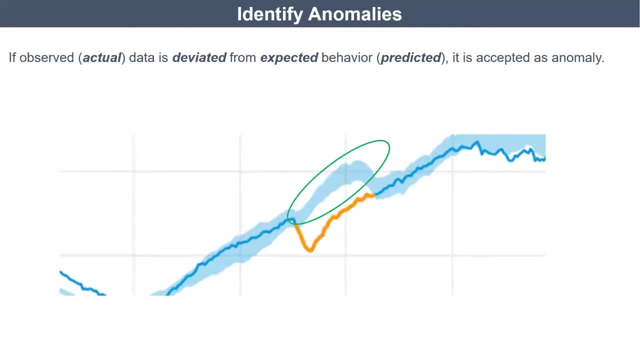 um, it's also um sort of defined as like: if um based on historical data, if we have some uh expected behavior, uh, so if our model learns the uh historically not labeled but historically known uh as normal data and if it is expecting such a behavior uh, and if our behavior, if the actual 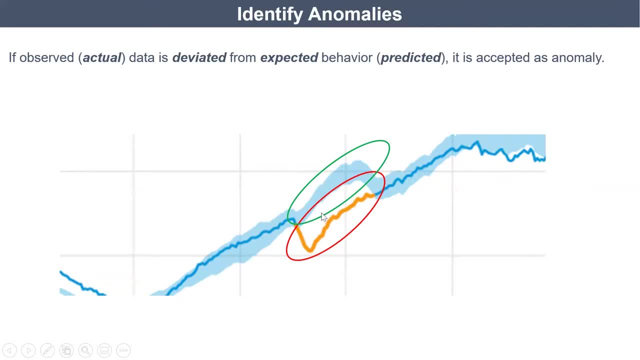 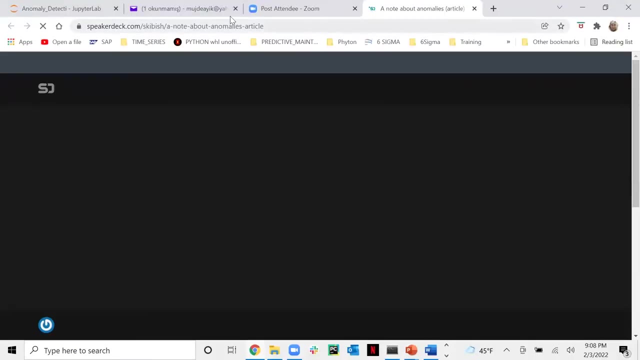 observation is not the same, then it's not the same. and if it's not the same, then it's not the same. and if the observations are different than the expected behavior, uh, within some confidence in trouble, uh, then we also call them as anomalies. so there's a nice link over here. uh, just to see if 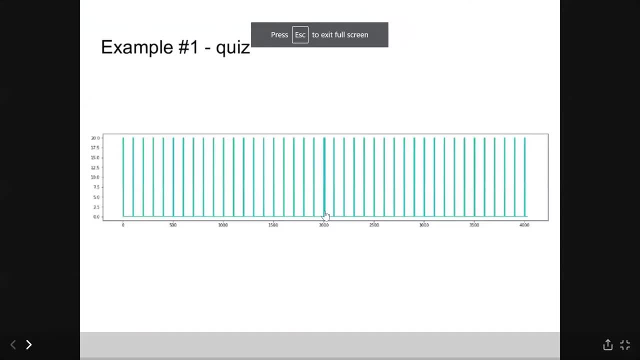 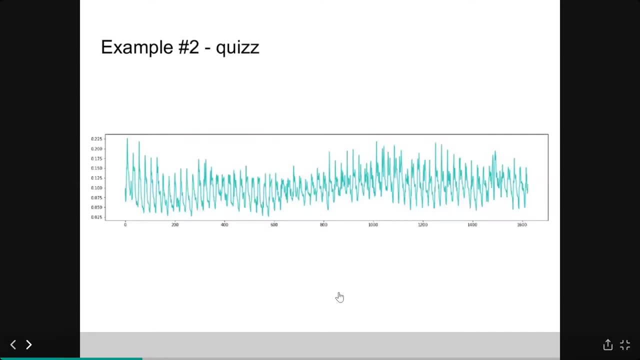 we can identify anomalies by eye all the time. uh, here it looks like i don't know. it looks like anomaly here to me. uh, which is correct? i haven't memorized the answers right away, i'm just looking. uh, but here it is more difficult to identify. 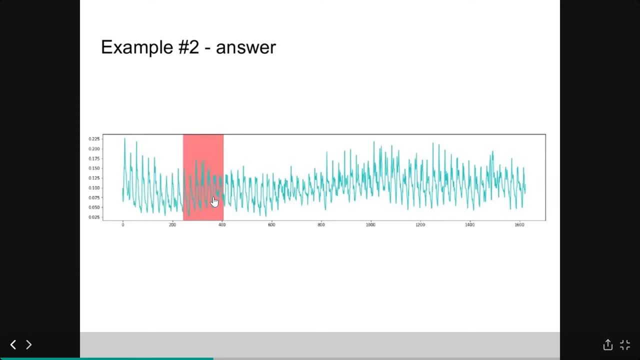 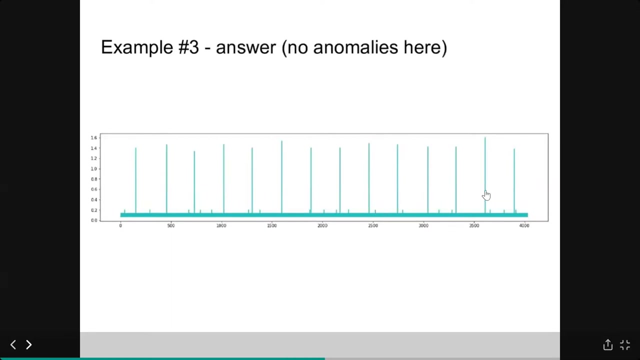 uh, maybe here, i don't know. no, i'm wrong, it's here, so it's difficult. i mean, in this case it's really almost impossible to visually identify such anomalies. uh, here, um, here, no, there was no anomaly in that one. okay, so here, um, i'm not sure what's going on and i'm just trying to get to the things that i just said here. 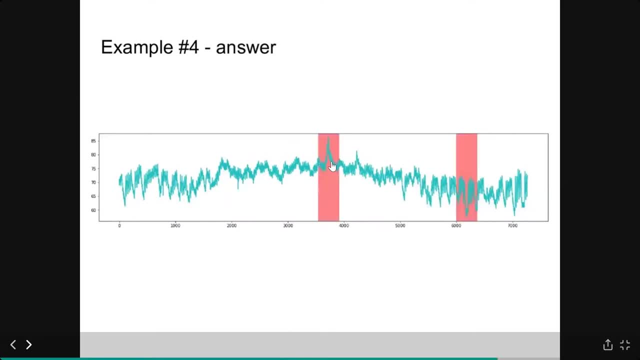 Here, perhaps here, yes, here one, and there is one more here. So possibly the model is learning the periodicity of the signal and the trend of the signal and because this behavior is not matching with the expected behavior, they are labeled, they are identified as anomalies. 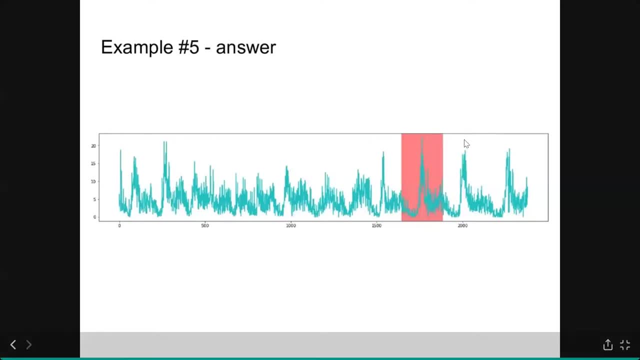 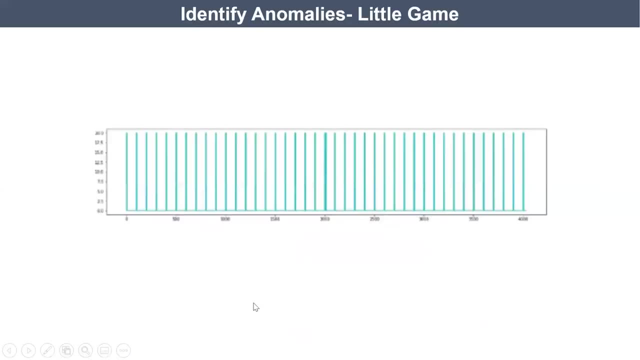 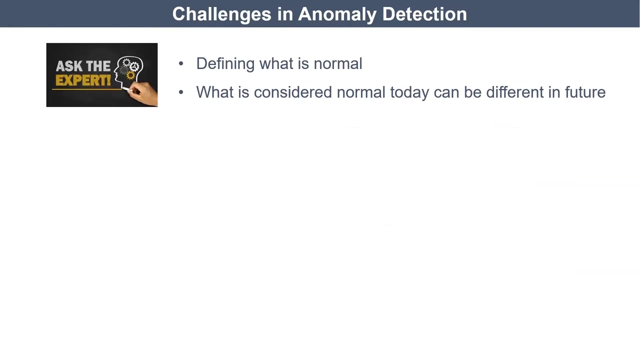 And this one maybe here. yeah, looks like it's here. So I mean here. basically, I want to show like it is not always that easy to identify especially multi-dimensions, and especially if the signal has some periodicity and some trend. it's not very easy to identify them by visualizing the data. 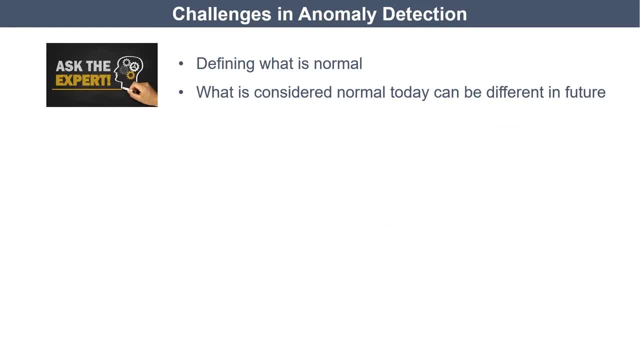 So challenges is basically defining what is normal. Normal is challenging because I mean today something can be normal but tomorrow it can change. Think it like, for example, if we are looking at customer behavior and we are looking into like fraud as abnormal behavior, today's customer profile may be different than tomorrow's customer profile. 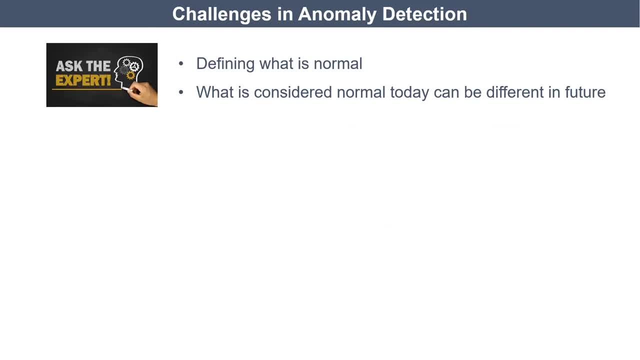 Therefore it's important that once we train our model on the normal behavior, So it's generally good to check if it is working okay and it is generally very likely that we need to update our models with incoming customers As usual, sufficient number of training and validation data set is important, especially- maybe this is important when it is unsupervised, because generally these events are a lot more important than usual. 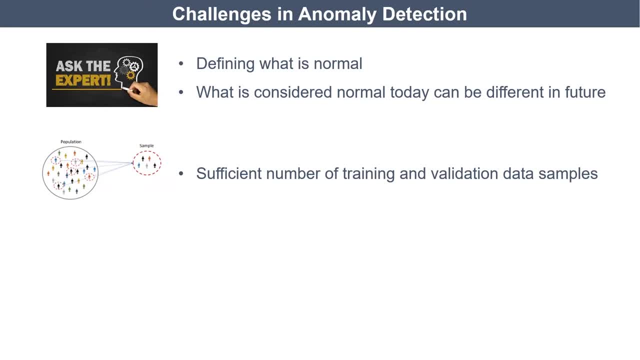 Like in fraud, are very rarely events, so it's important that we have got a good representation of our data. It's important that we have got exploratory features- sufficient number of features- and we need to be careful of high dimension space, as I mentioned. that's challenging. 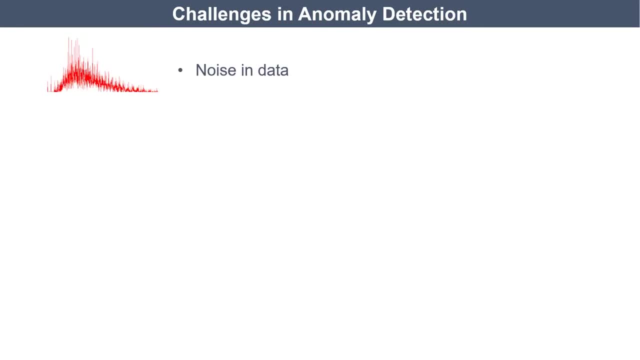 Noise in data is really important. I have experienced that myself as well, because we don't really want- I mean, once we get our basically um data from sensors especially- uh, it's impossible that it's not noisy, so there's always noise in. 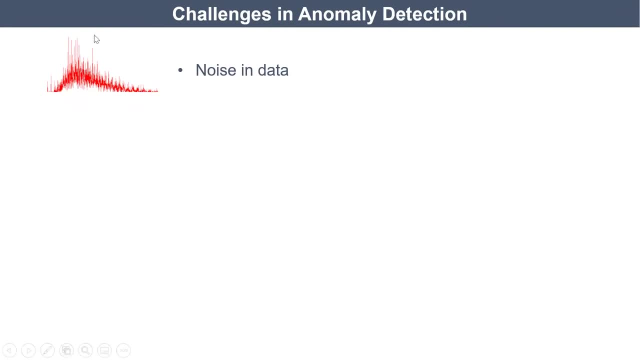 data, but obviously we don't want our model to learn this noise as well, uh. so, uh, at that point actually, uh, in my experience, we were coming together with field experts and we were trying to um filter that noise before we feed them into the model. but i mean we should filter in a way that 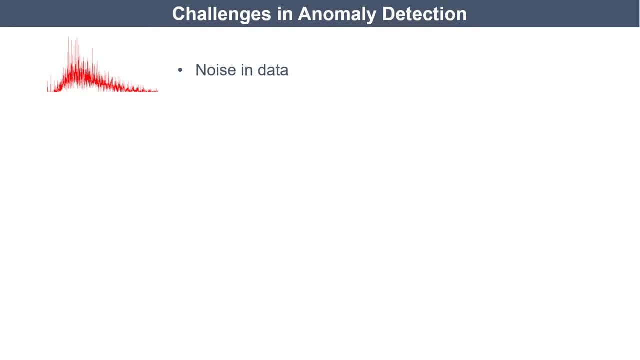 that shouldn't cause any lack in the response uh. so, uh, at that point, really, uh using a proper filtering approach uh and uh getting coming together with field experts is very important uh when it's a time series problem. um, short time series uh is challenging uh, because i mean the 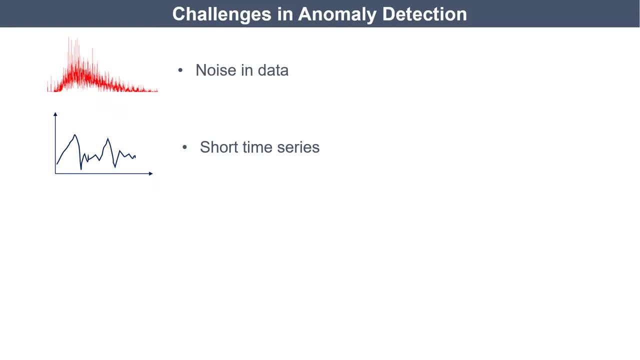 model doesn't have too much to learn, but on the other hand, if it is, i will show some examples. if it is like different vehicle rights, they are all short rights. we need to find the way to combine them because basically it's not a long time series but we have got many short time series at hand. 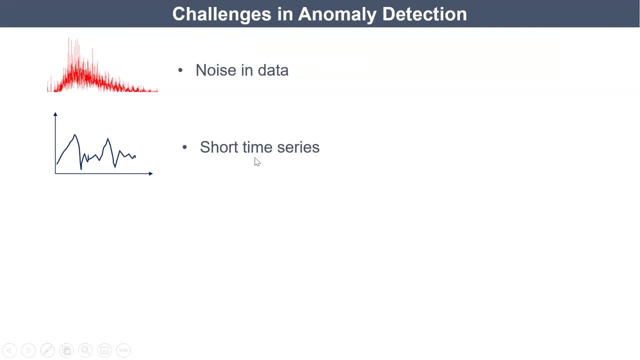 so we need to find a way to um sort of combine them and i will show an example to you. in that importance of data processing is really important in terms of features and, as i said, like in terms of cleaning the data and stuff like that. um, and here, 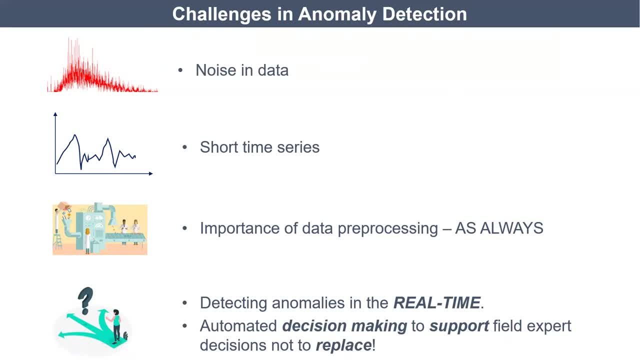 uh, detecting anomalies in real time is really challenging and uh, in my experience, people are generally do not solely rely on automated decision made by the models, but they are generally used to support decision makers in the business, which makes, i think, sense, uh, to be on the safe side. 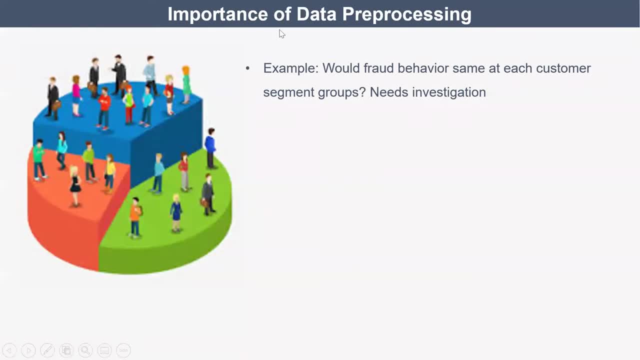 uh importance of data processing. an example could be like, for example, if we have a customer segmentation that we have already done on customers, maybe using k-means, clustering or demo in terms of demographics and, uh, basically, spending behavior of customers, we have different segments of customers and if we, let's say, want to develop a fraud model on this, 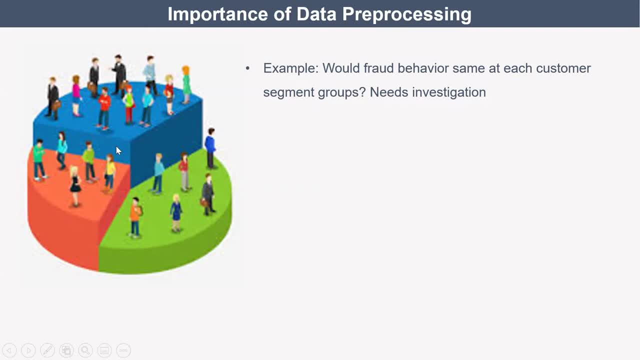 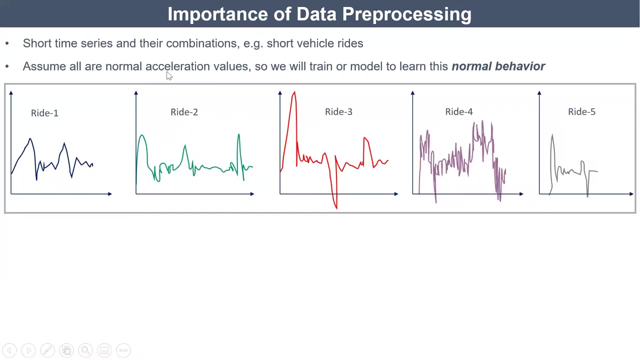 uh, we may not. we need to investigate because, uh, one model may not work well for each segment. uh, because their behaviors may be different. so, uh, we need to, we need to test, uh, different, um, basically models for different clusters in the data short time series like this. this it was like one of the examples i found very challenging when i 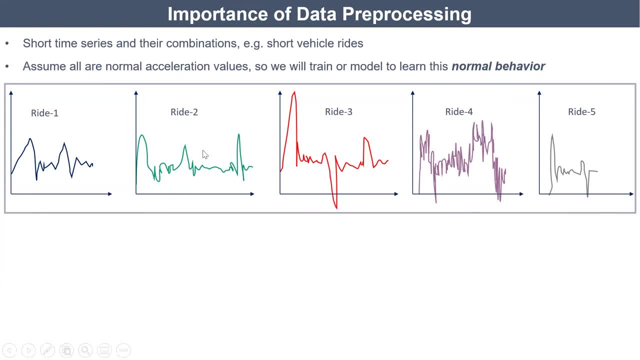 was working for um, um, basically health monitoring of flights in mississippi. so we, we like, in fact, these 3 to 4 hour 플� g show. uh, nowadays, you know, on doctrine of coveting flights, a flight every 18 days and uh, we have been particularly trying to the transport climate. 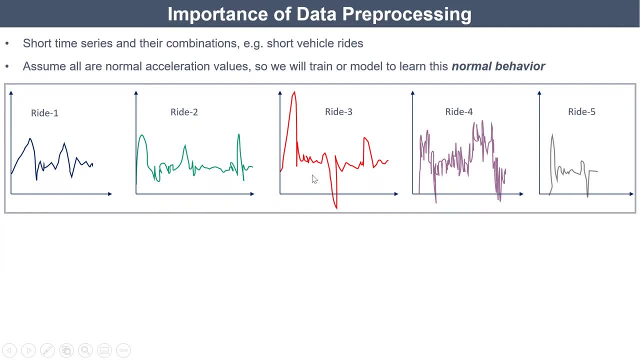 and so we, we 우리가- used older vibration rondelle revolt, so we knew that when theو So uh, when uh it is believed that the Manchurian a liver hear could mean total right, um, so so uh. there there are a few cases where um occult information and uh. 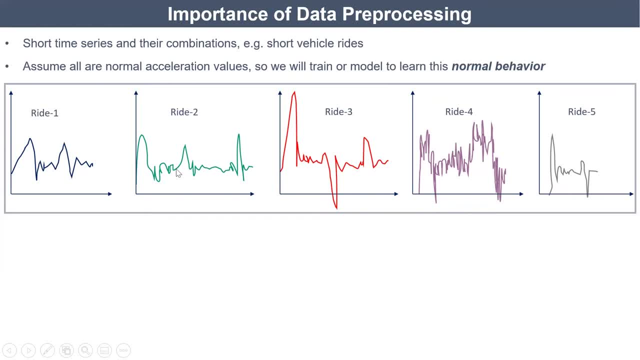 uh, so we used two product. of course, the хочет does not provideiler light�, um, so uh, asics does not supply any uh� keywords, Russian. you know, for example, that in order to obtain gosh, uh, if this light, then as they can't control them, so so, basically, so like in terms of, I guess, k스� which배enses which. 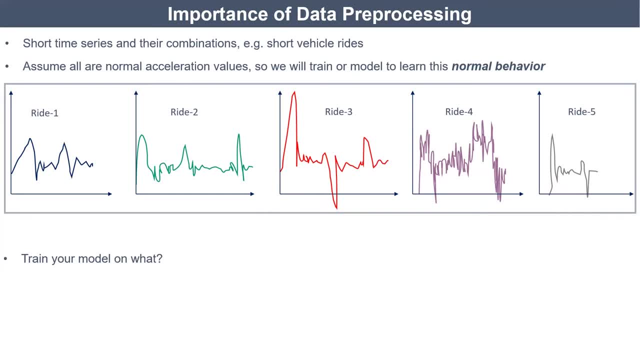 need of purpose, recorded this. it's okay to basically rely with uh. we basically rely on uh, the field expertsinhasha. when we have many rights like that, how could we train our model to learn the normal behavior, uh, normal acceleration behavior, uh, can we like train uh models for each right separately? 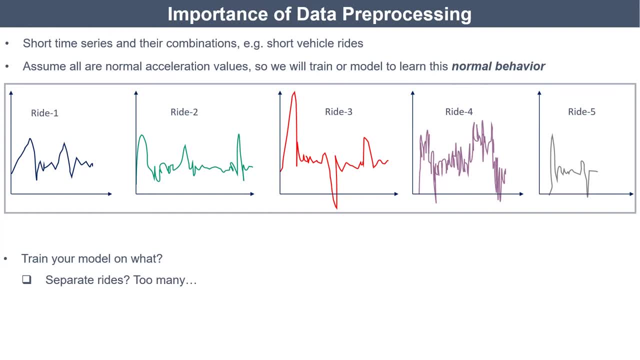 uh, which doesn't seem very reasonable when we have too many rights, and how we are going to combine them. um, can we combine the rights? uh, just one after another. well, we need to be really very careful in that, because we need to find a method to tell the machine learning model that this, this, 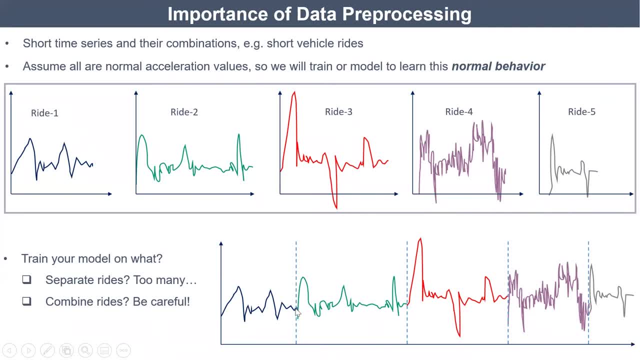 part. the second right is not the uh continuation of the first right, so at this point we should tell the model that this ride is finished, so just mask down values and another right starts again from here. so, uh, basically, our models should learn that each of them are separate rights. 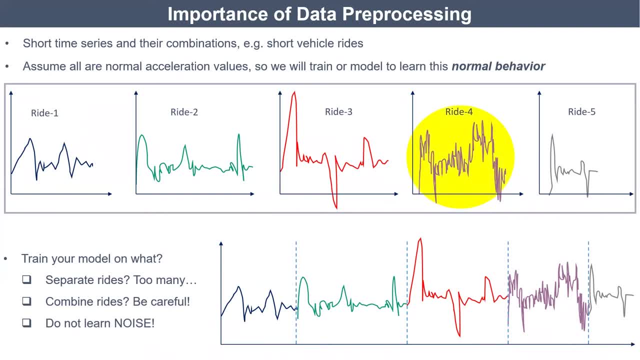 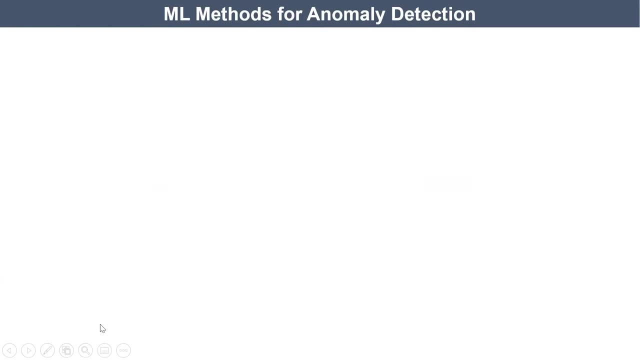 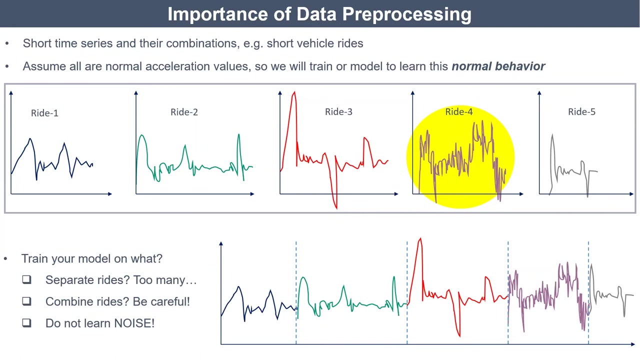 they are not following each other and important thing is that, as i said, we should not learn noise, so we should feed, feed uh filter data in our models. uh, i had really similar curves uh with photodiodes from robotic arms in a factory. they were collecting sensor data and they really look like this and 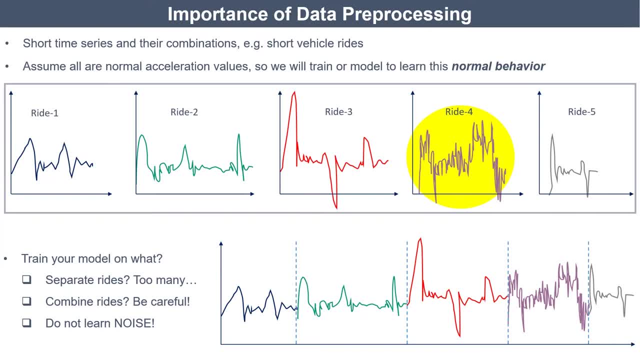 i mean in sensor data, i guess it's quite common. yeah, i mean noisy data is very common when we have sensor data, uh, but i mean that's why, really, data processing is very important, uh, to find a good filter which doesn't lead any lagging response. 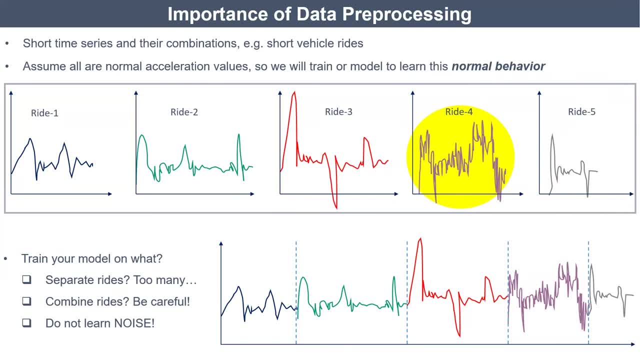 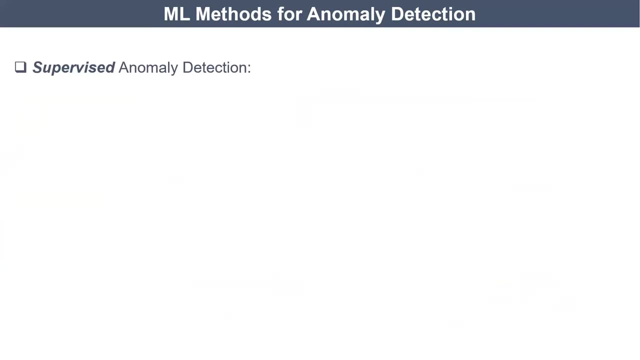 and uh. smooths are um, basically signals, uh- in a sufficient way, i would say so. after that, we have the basic data collection and we're gonna get good quality data and all the other things that we can use in order to create a better quality data. so let's see if we can integrate any of these uh, our kind of, you know, automated data. 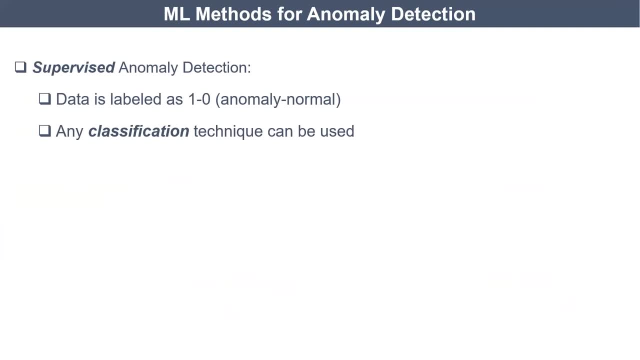 can i move on? yeah, thanks. uh. so if our, if we are lucky and our data is labeled- which is almost impossible in time series data, um, but maybe some tabular data, um, But we need to be careful about imbalanced data sets in this case, in terms of two things basically: maybe in terms of performance measurement metrics of the model and also in terms of sometimes people do upsampling or downsampling methods to basically get rid of this imbalanced data set. 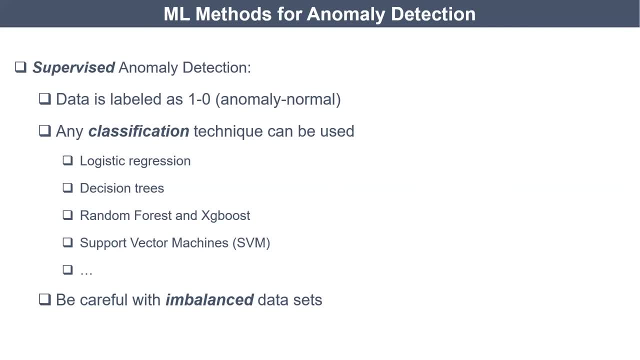 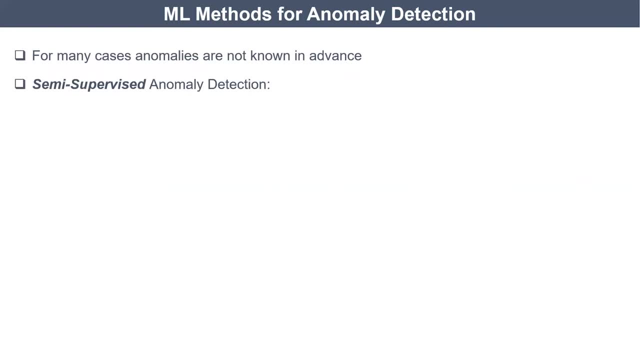 which is very typical in fraud as well. For many cases anomalies are not really known in advance. So we have got also semi-supervised anomaly detection. Again, there are no labels, but at least we know that our training data consists of normal. 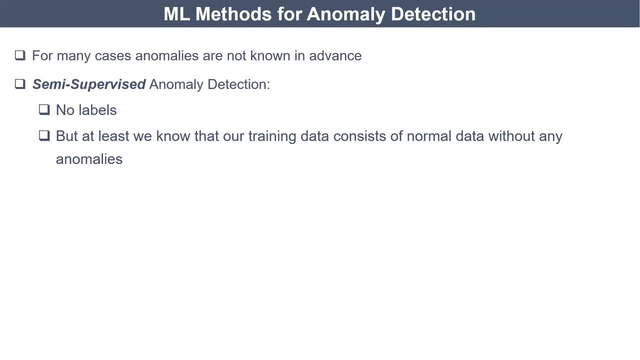 data, I mean our field experts come to us and say: okay, just basically train your models on those signals. We know that physically Those rights were okay. So once we know that there are no anomalies in the training data set, then we are happy. 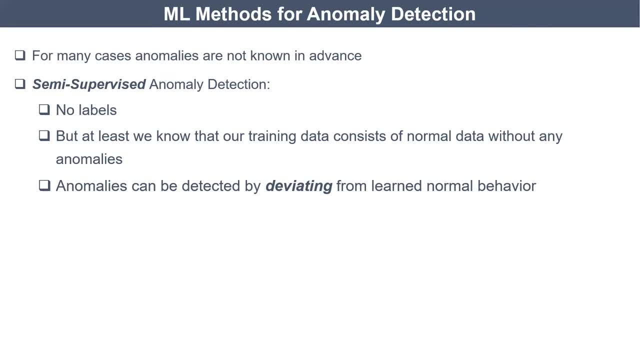 In that case we basically train our model on healthy data, on nominal data, And then we detect anomalies, basically once the observations are deviated from the learned data set. So that's the first normal behavior. I'm sure there are many more methods, but the ones I used- not all of them I have used- 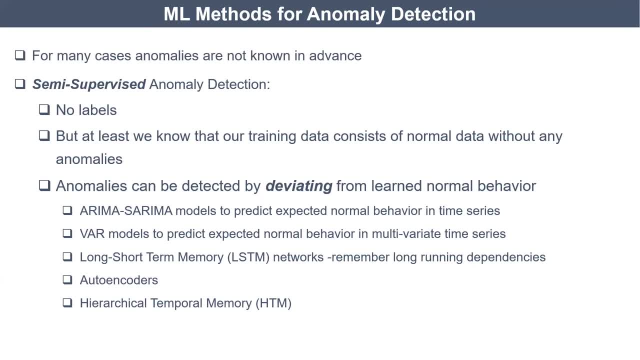 but LSTM like deep learning, basically a deep learning method to remember long-running dependencies, especially in time series. LSTM, autoencoders, ARIMA, SARIMA and wire models to predict expected behavior. So that's the first normal behavior In time series and there are HTM models as well, which I haven't used before. 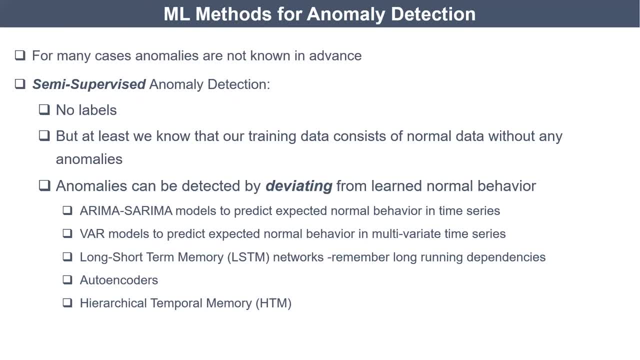 But I mean, the idea is all similar because they are basically assuming that data is normal, Even if it is in multi-dimensional space. they are basically learning the time series dependencies so that we can expect- we can sort of learn what to expect from upcoming. 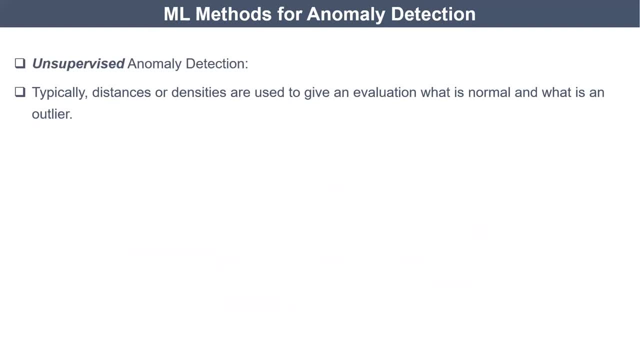 data. There are obviously unsupervised anomaly detection models and these methods rely on distances and densities generally, And the methods are rule-based approaches, as I mentioned before, like the interquartile range method, standard deviation method or histograms, but they are generally suitable. 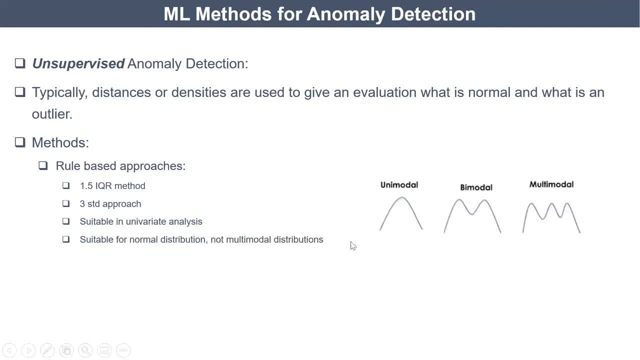 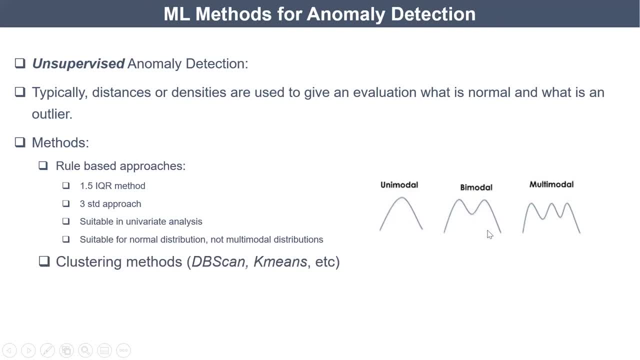 Robyn N個al, And there are also other density based techniques: Canier needs, neighbor look, lot, life factor, isolation for SVM and there are many more. actually, Bayesian networks are also youth minimal selection. But For this basically presentation, I will be� 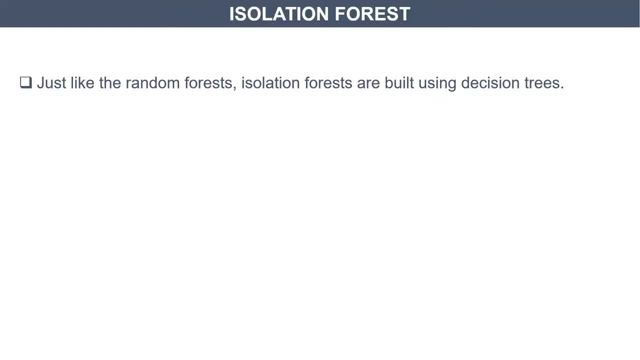 I wanted to focus on one of them. I think the semi-supervised ones are also important, based on the time series prediction ones, But that's more a deeper subject. Maybe we can discuss on another call. It's a little bit more detailed. 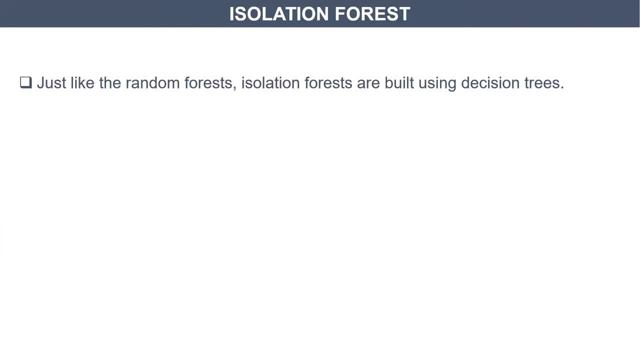 Isolation forests are basically? they are like random forests And they are built using decision trees. They are implemented in unsupervised sessions because there are no labels. Basically, it's just like random forests. It's again an ensemble of trees. 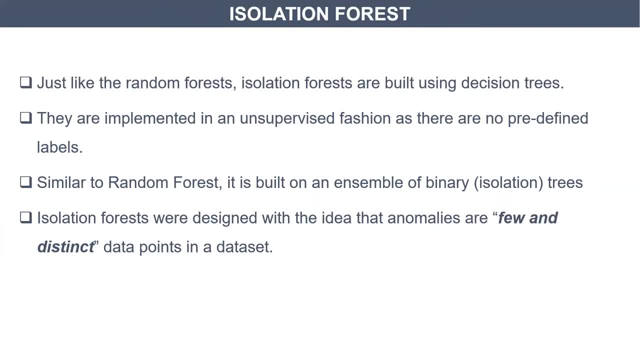 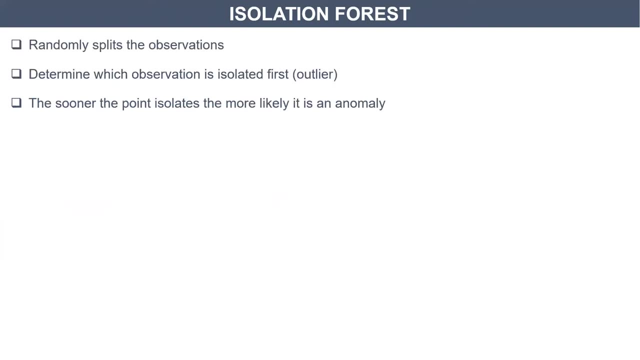 And the assumption behind is that anomalies are outliers And there are really few distinct points so that they can be isolated easily. So the assumption is based on that. So it basically randomly splits the observations and takes each point and basically finds the number of steps to isolate the point. 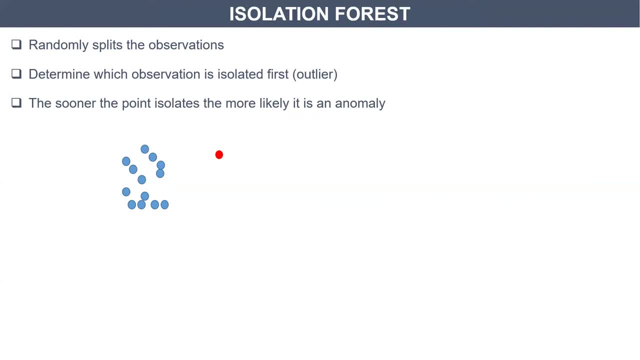 So the sooner the point isolates, the more likely that it is an outlier or anomaly, Like for example in this case. if we have a split from here and one more here and one more here, we can easily isolate our point. 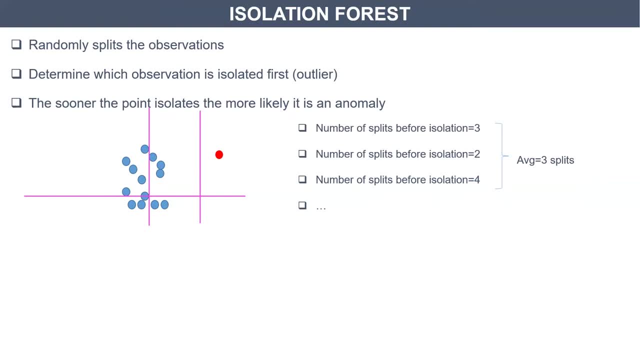 And in that case we would say: OK, in random, many different splits, in average we could get to this point, isolate that point in about three steps. But if it iterates through this point, I mean if it just tries to find the label for this point- 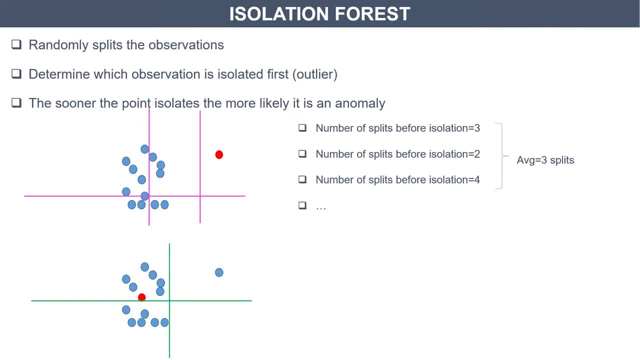 then it will take more steps, obviously because it's not as isolated like the other case. So in that respect, number of splits would be much higher than the previous one. So once that number is much, much lower, then it's more likely that this is an outlier. 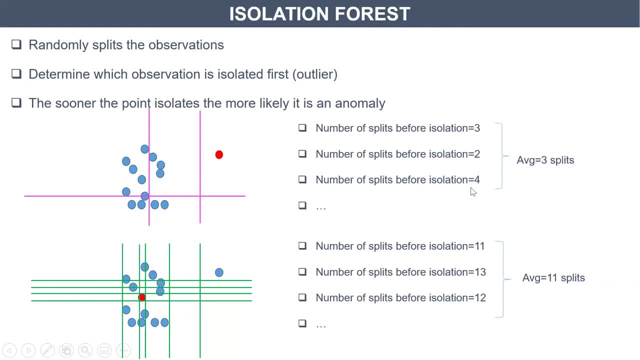 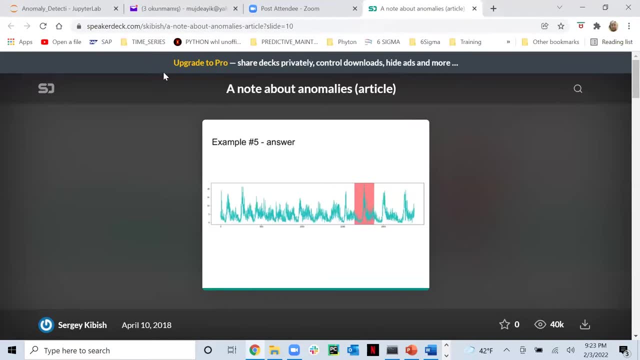 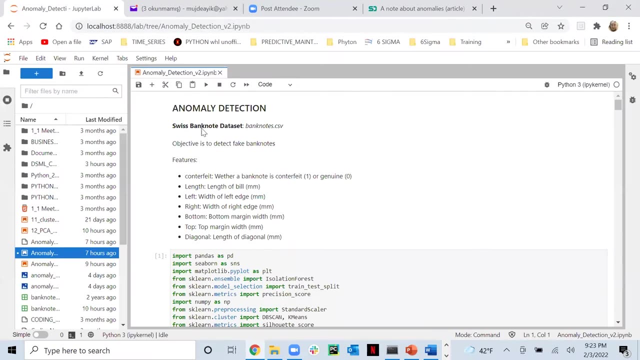 or this is basically an anomaly, So the idea behind is that this one. So I just have a notebook for this, OK. So basically, I have used this Swiss banknote data set, which has got these features, basically, And we have got a label, but this label. 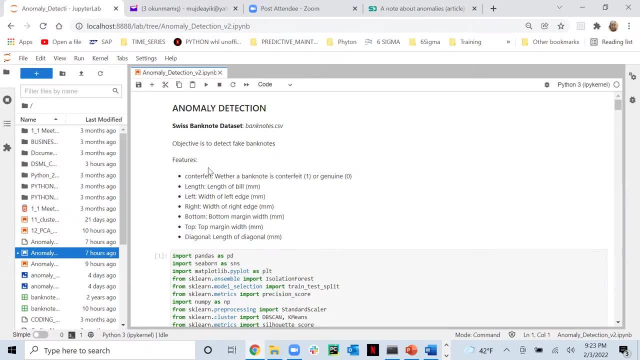 is just to double check ourselves. We are not going to do any classification in that respect. We are just going to basically test our unsupervised approach here. So basically, this feature says, like this banknote is, take one or a genuine one. 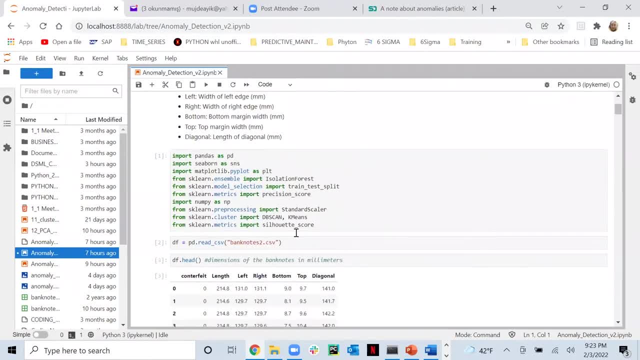 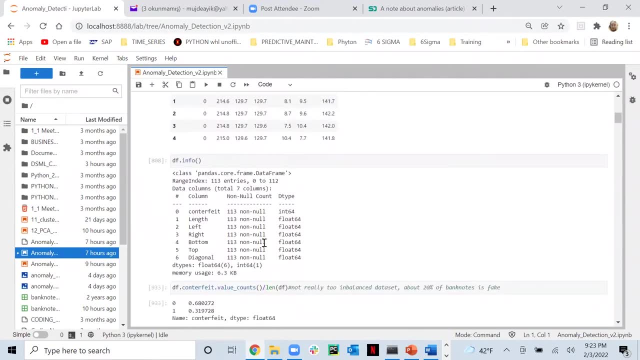 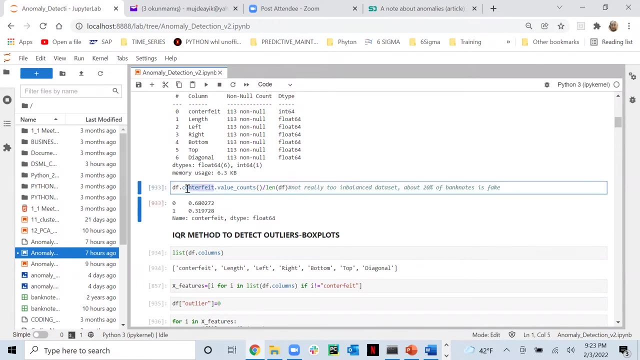 So this is a little bit modified version of the Swiss banknote data set. So we just read through this data And it doesn't have too many features anyway, And once we look into the sort of the counterfeit, when you can't, it's about like 32% of our data is, I would say, fake. 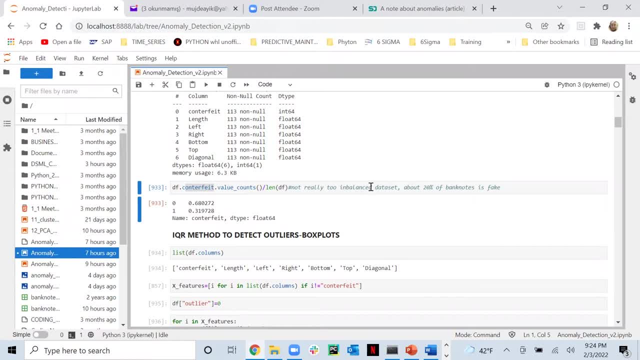 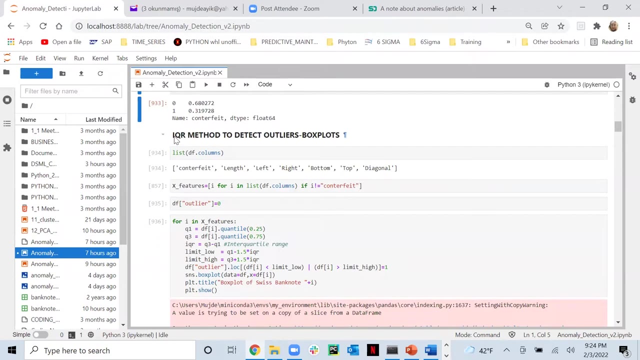 which is not really too imbalanced in that context. But there would be cases which could be like 10%, even 5%, which we would approach differently, maybe up-sample or down-sample the zero cases. So if you just simply look at the entire quartile range, 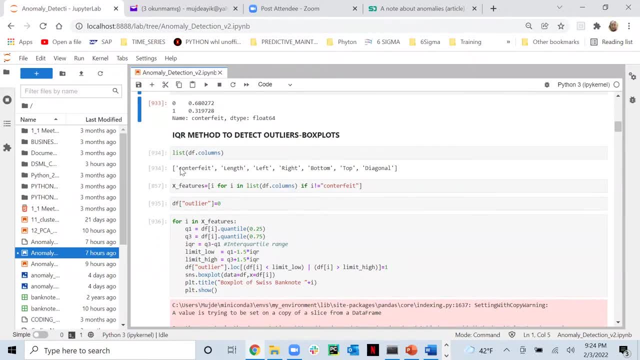 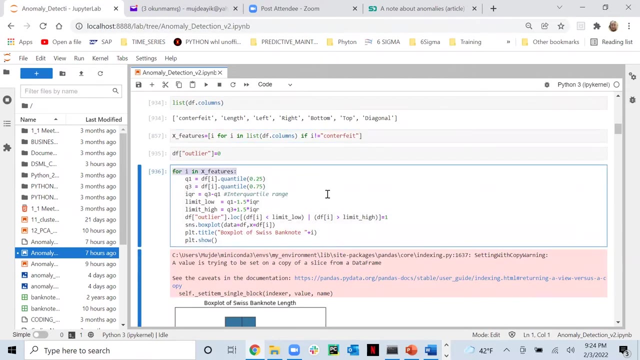 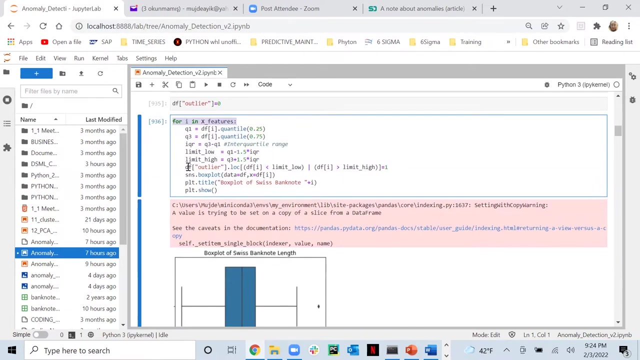 method to detect outliers. basically- And this is our X features- dimensions basically left length, right, bottom dimensions. OK, So what I'm doing is here: basically I'm looking over the features and I'm getting the low and high quartiles limits. 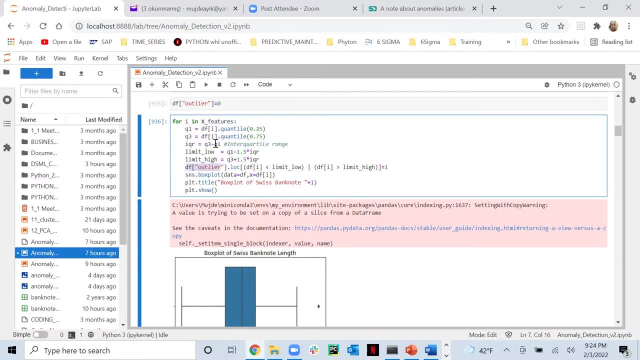 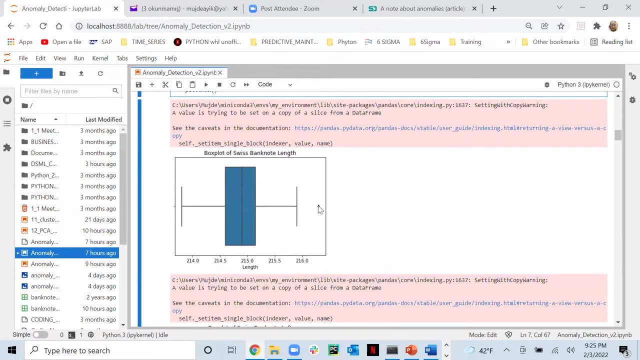 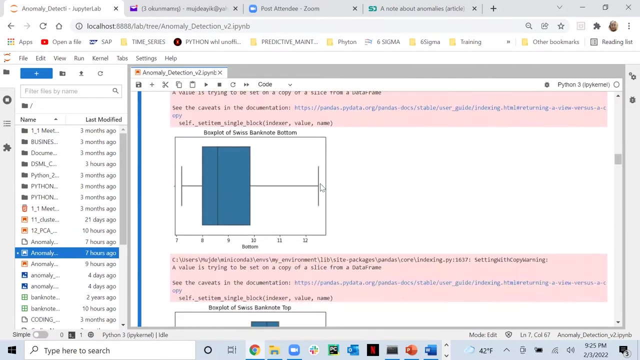 And once the observations are beyond those limits, I'm basically labeling them as outliers here or as an anomaly here. And once I basically plot the box plots, I see that there are these outliers here. These are visually easy to identify, especially in one dimension like this: 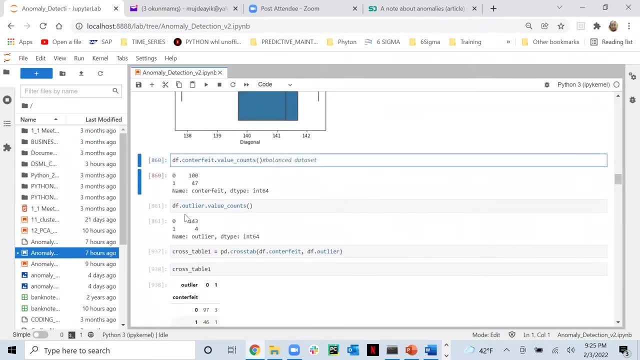 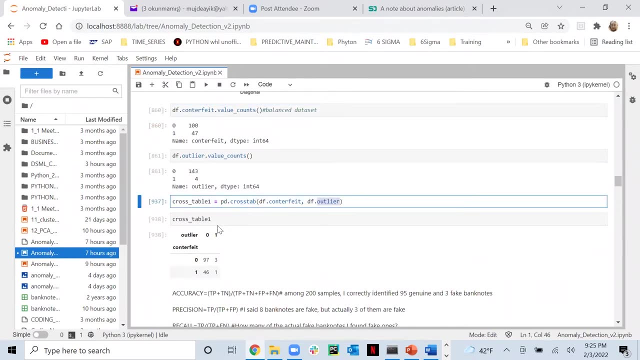 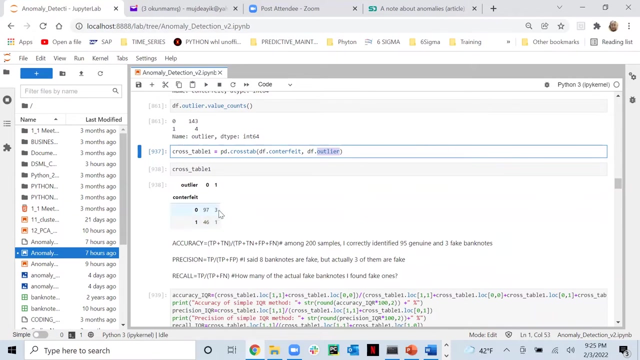 Then. so basically, what I'm doing here is then: OK, I have set my outliers. So if I look at the cross table between those actual values and what I have identified as outlier without using those labels, I see that. OK, these are my true positives and true negatives. 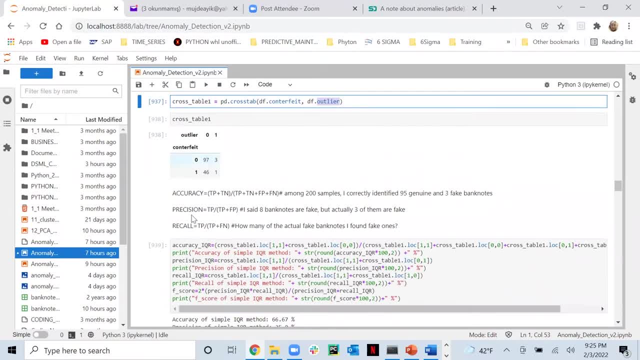 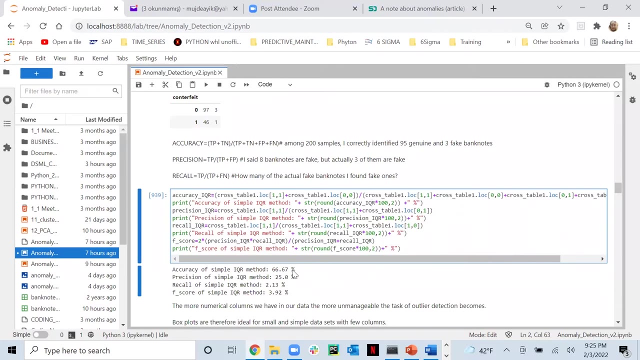 and stuff like that. So I'm looking at all accuracy metrics, all performance metrics mostly, And just to basically explain people better- maybe the students- I just use the formulations myself And only looking at the entire quartile range method, we get an accuracy of about 67%. 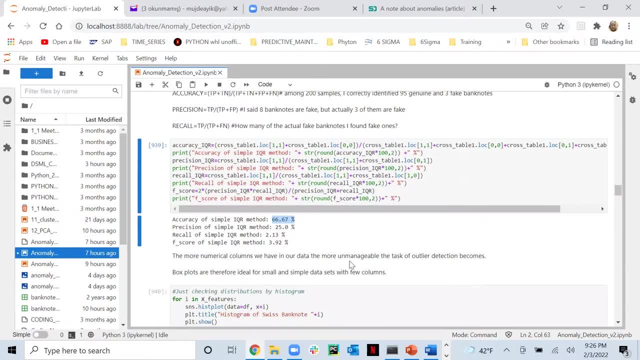 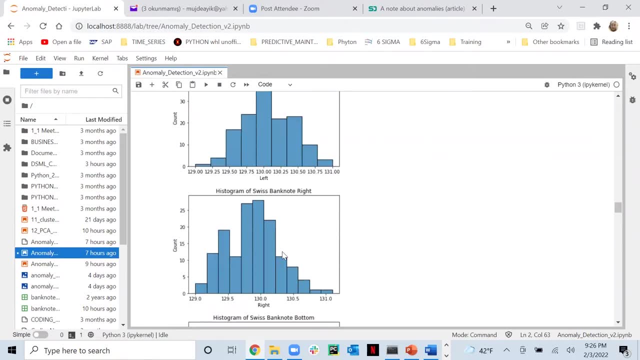 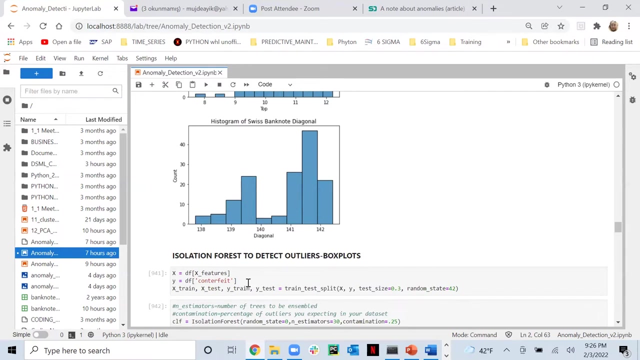 And here I want to also look at the histograms as well. I mean, this looks normal, looks normal, looks normal, Not too bad, I mean. but here, for example, these are like the model distributions, So I'm sure I can do better than IQR range method. 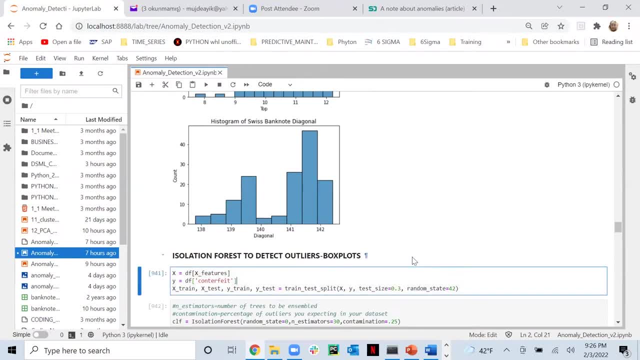 But sometimes these sorry Müşter, sometimes these IQR methods, histograms, They are more like the normal methods, or let's call them simple methods. They can really create miracles. Some people are really not familiar with these things And if you are on board to a project in a factory, 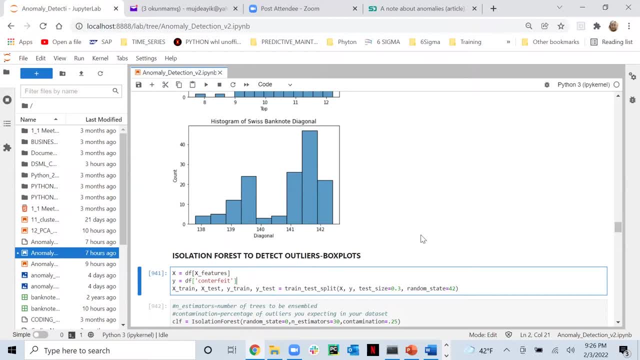 or in a company and they want you to do these kind of anomaly detection. And I guess this is as you are very well presenting. this is the first step to take. Yeah, First do the simple thing. Yes, I'm very happy. 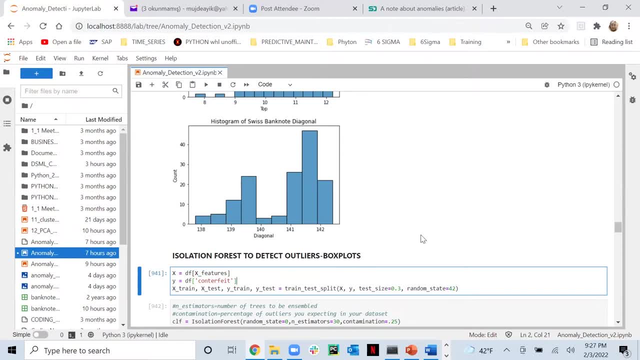 And you are 80% Easier, Yeah, And it is OK. But I mean it is OK to look into such things like in one dimensional stuff just visually understand what's happening. But in multi-dimensions, and if there, 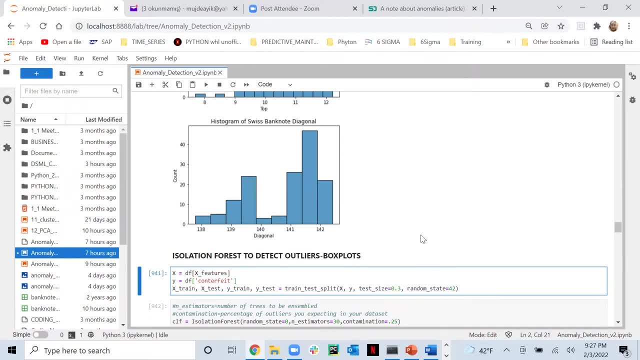 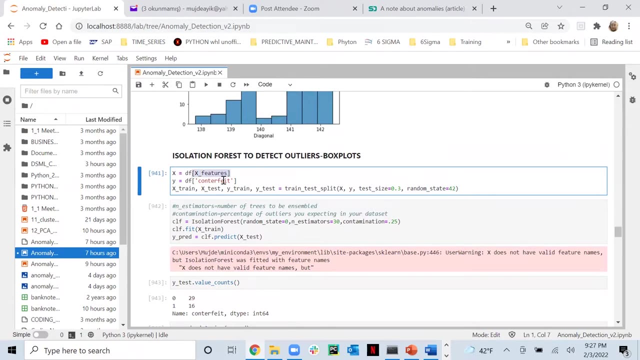 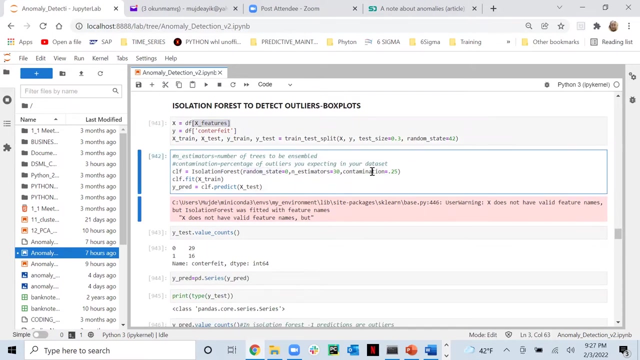 is a time series component, then they are not helpful in that respect. So we had about like 67% accuracy, Not too bad, And if you use the same data, if you use the isolation forest, training can test it basically. So there are some factors that you could play. 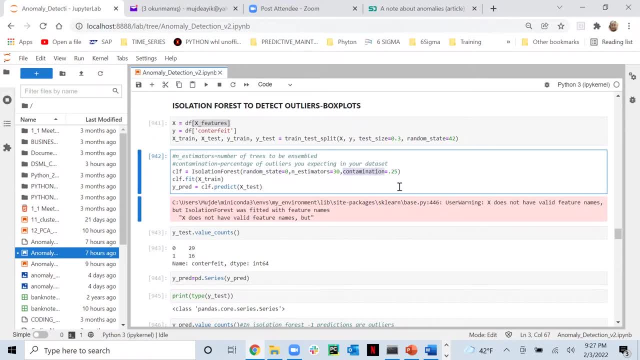 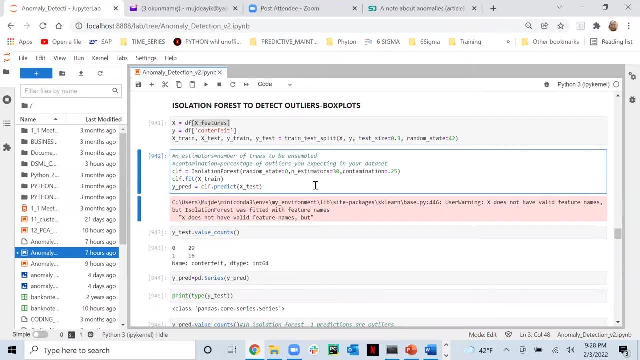 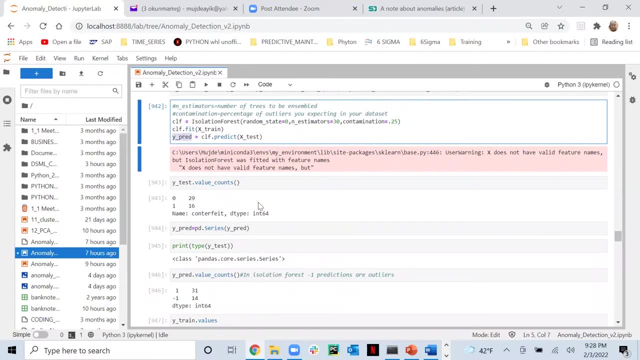 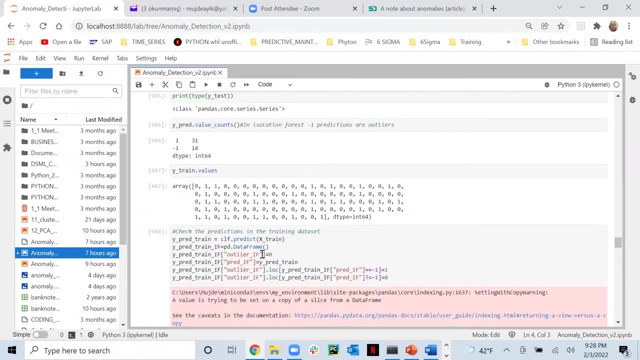 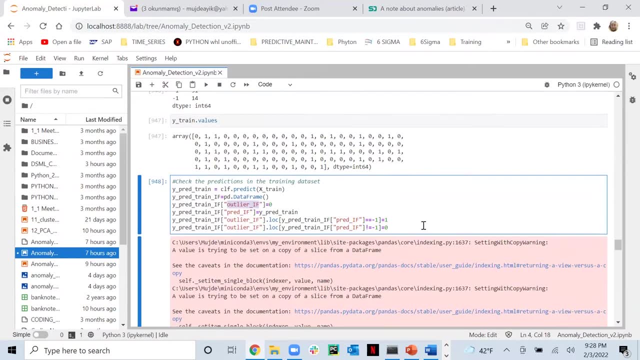 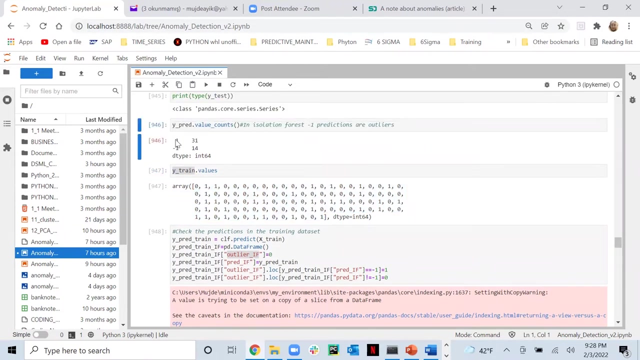 We do our prediction And basically then I'm just adding another column as identified outliers by this method, basically. So when I basically train this model, So I get labels as 0 and 1.. Actually not 0 and 1,, 1 and minus 1.. Here actually minus 1 means. 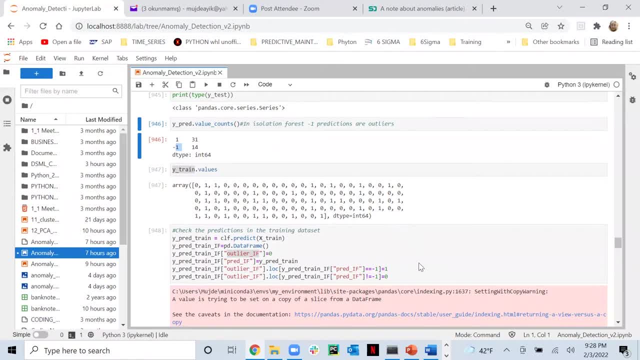 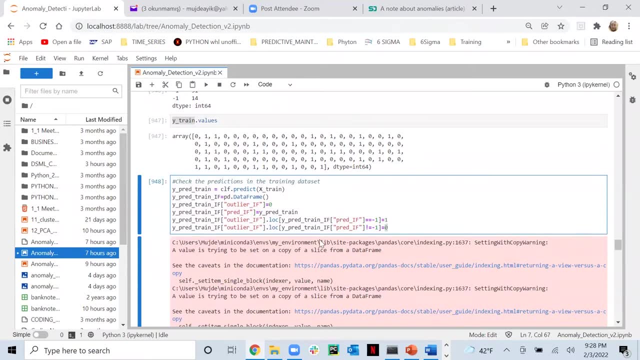 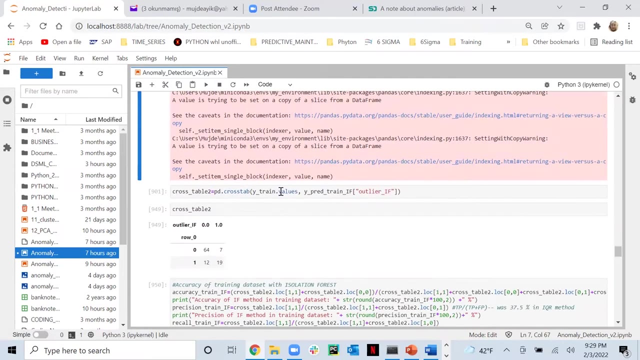 outlier. So to make it similar to my data frame: if it is minus 1, I say it is fake, And if it is 1, I say it's not fake, so that I can basically compare this with our actual labels. So looking. 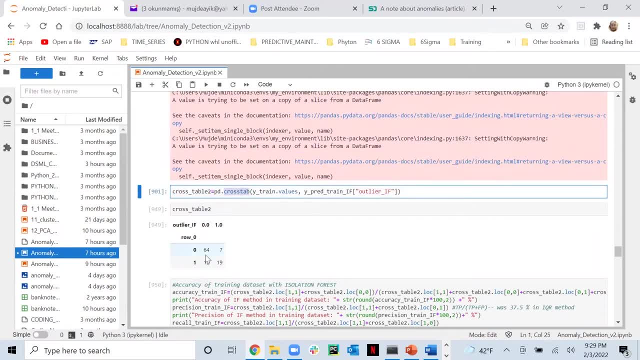 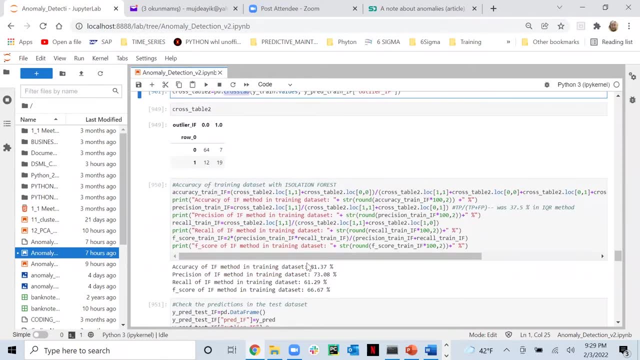 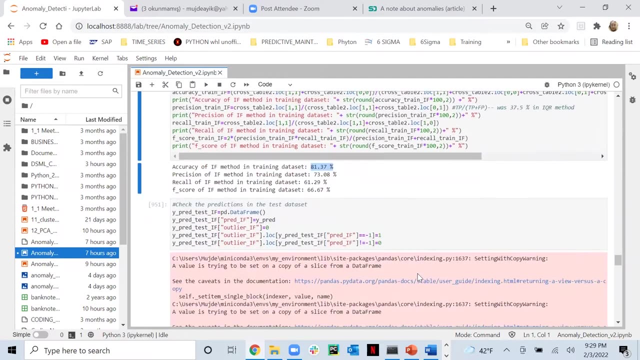 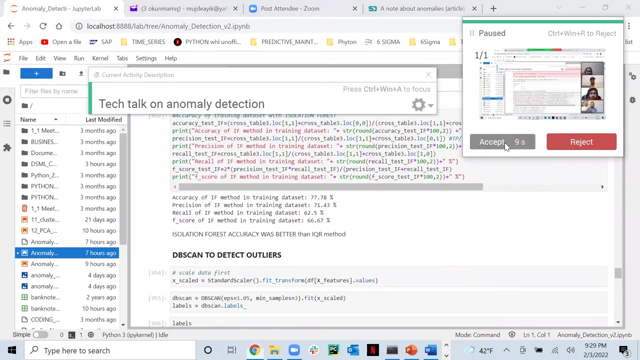 and comparing this with our actual labels. then I get this cross table And, looking at the accuracy of the results in the training data set, I go up to 82%, which is better than our simplest approach, And I do the same thing on my test data And I get about again 80%, 78%. We could do some. 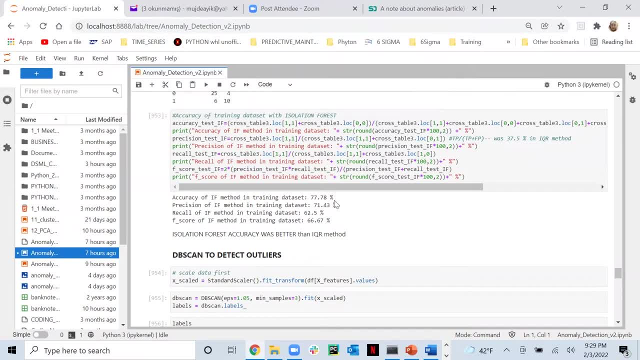 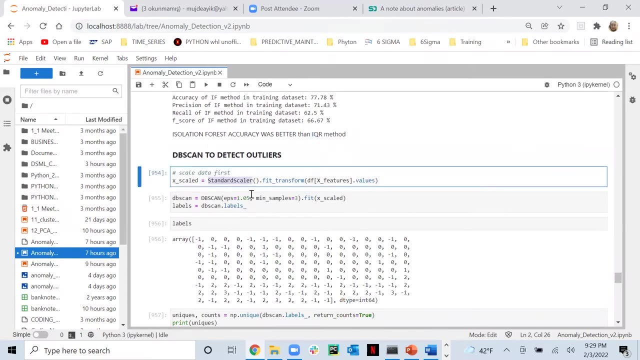 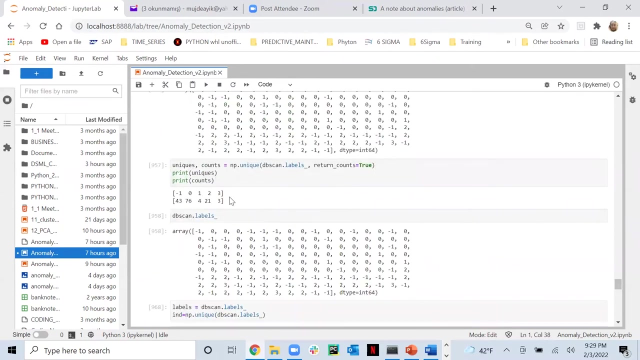 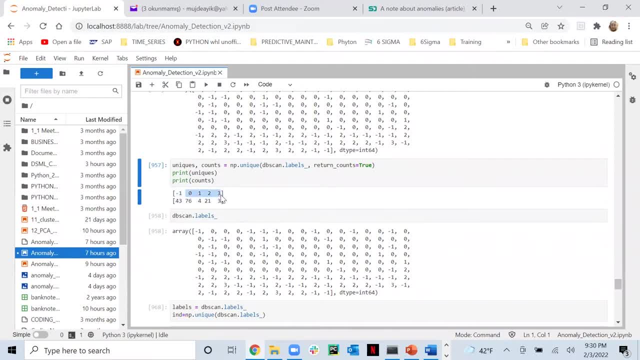 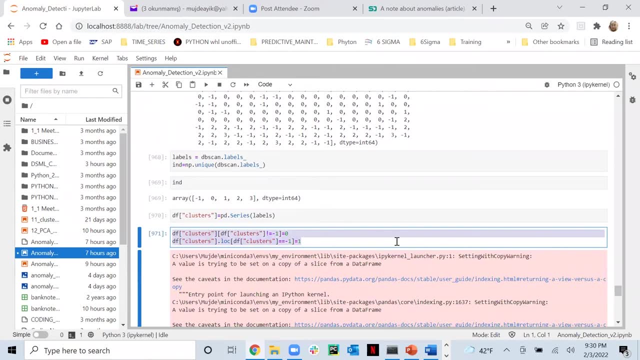 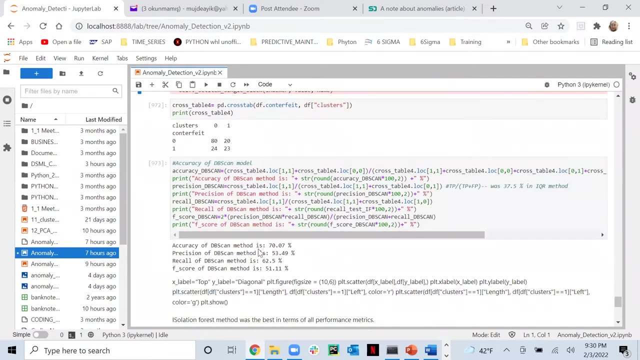 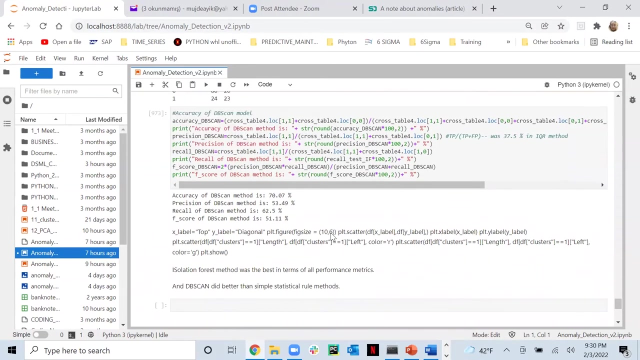 outlier And when it is not minus 1, I call it as basically a genuine banknote. So I just mention it here. And when I look at the cross table here then accuracy is another stuff. I see that I get a 70% of accuracy in my outlier detection, So overall it looks like isolation forest. 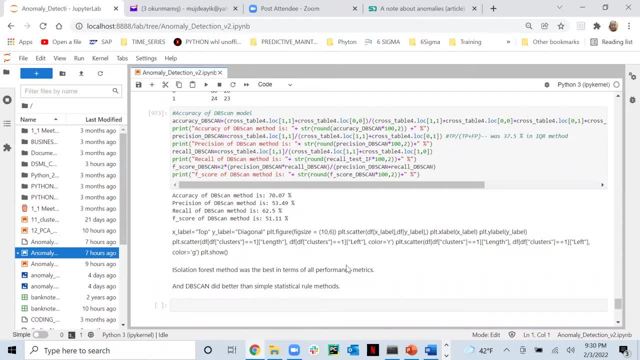 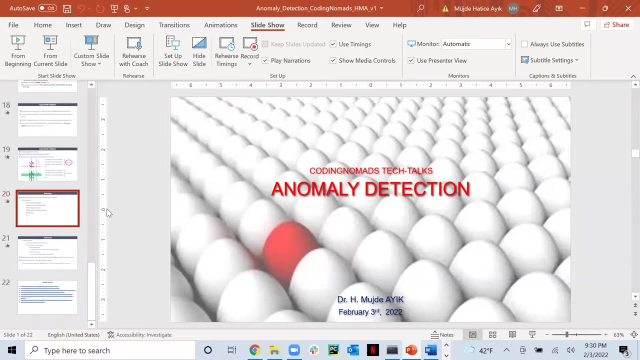 was the best in this analysis in terms of performance metrics, And dbScan again did better than some statistical simple rules. There are many other methods that we could study And really the approach to the time series is totally different, But that's really another subject to go over. And finally, if I need to summarize my points, 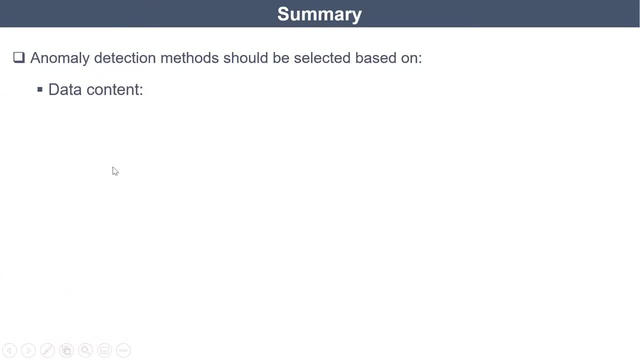 I'm going to go back to the data content. So a number detection method basically should be selected based on the data content, if they have got any time component involved, if it is univariate, multivariate analysis. our feature dimension space. is it supervised or unsupervised? 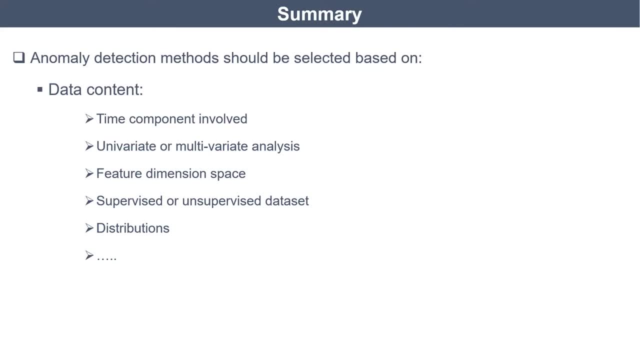 or somehow do we have got like a known normal data, like in some supervised case? we need to look at the distributions. Field expertise is really very important because they physically know what is normal behavior, So they know what to expect as normal. So we need to come together with field experts And before the 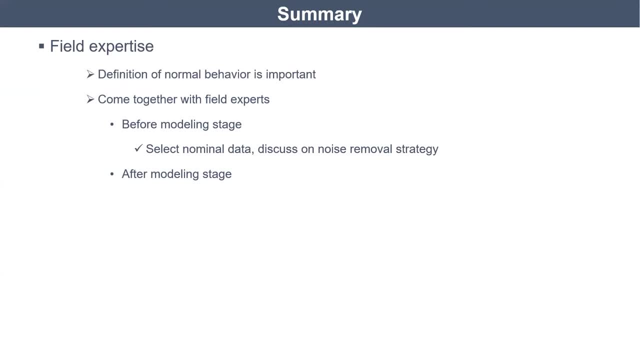 modeling stage to select nominal data, healthy data, discuss on noise removal strategy and stuff like that. And after modeling stage again we need to come together and look at the data content, say, Okay, these are my predictions for anomalies, they make any business sense? or physically. 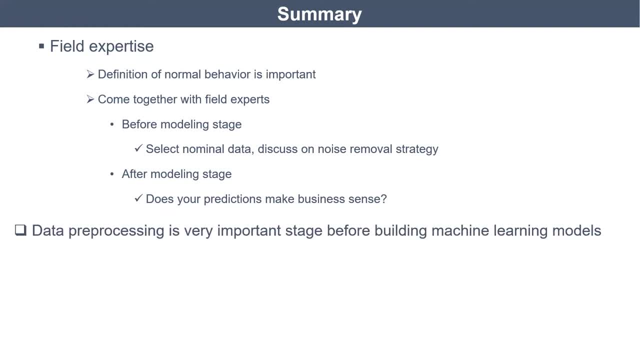 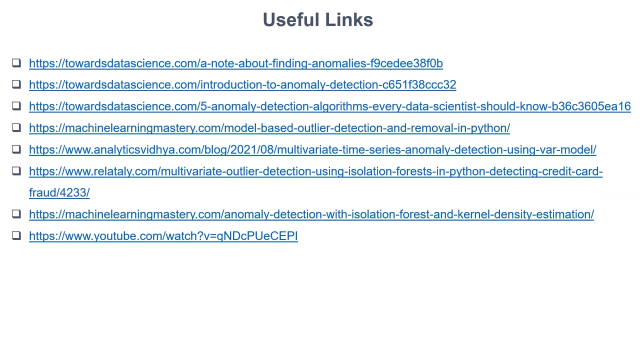 are they reasonable, kind of thing? And data processing is really important, as always. And again, if you are doing real time detection, then we need to be really careful to be on the safe side. So that's all from my side. if you have got any questions, I'm happy to answer. 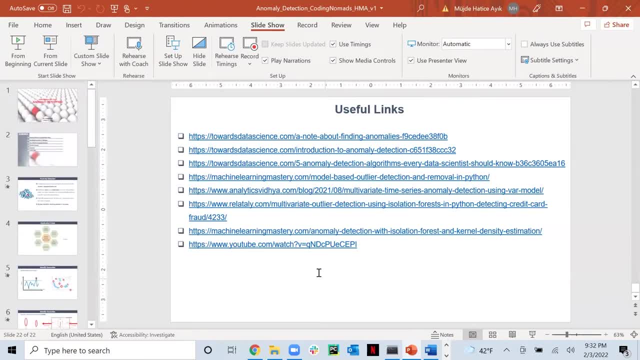 How many questions is a good? is a is a good question? I have many, But thank you so much, Marisa, for for sharing all that. It's fascinating stuff, I think. honestly. one big question that I have is, given that Swiss banknote data set. 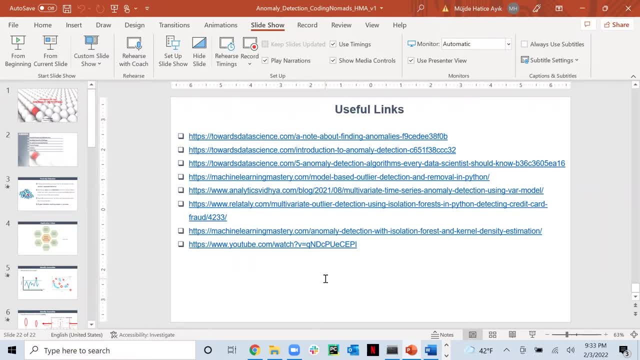 What would the recommend? You tie it together for me as the what's the final product And how does in? in those three examples that you had, and let's say, let's take the isolation for us, which was the best, What now? Now, what like? how does, based on that, What is our? Can you basically explain? 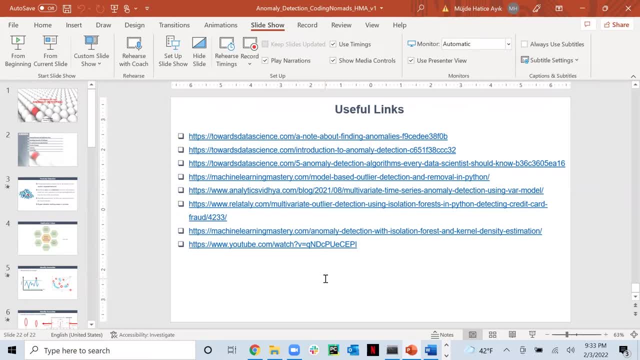 the final result from the- in the best case, the isolation for us, and what that actually allows us to predict or forecast and how that would be useful in the Swiss banknote sense. That makes sense, Marisa Peerishis. I mean Swiss Banknotes, I mean it's. 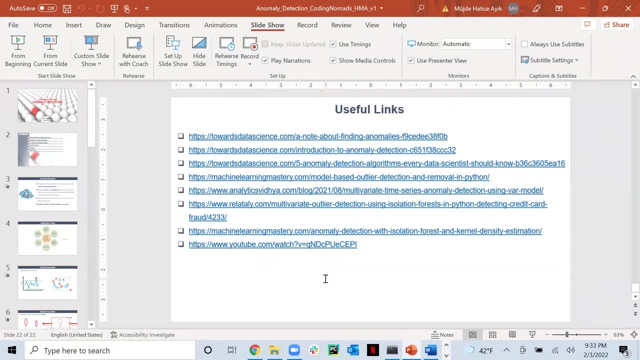 And I'm not very familiar with the subject, but I mean, maybe I could give an example from my experience, Like, for example, when we were doing predictive maintenance for flights for GE engines. basically we were identifying those anomalies And we were saying we were using Bayesian networks. by that time 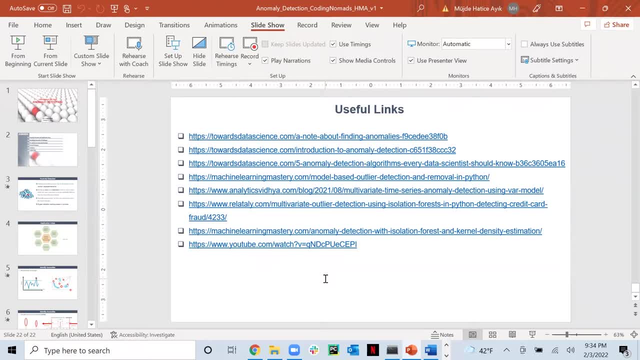 But anyway, we were saying like daily we were getting all the data and looking at the data and feeding them into the model. We were saying like OK, there is a 75% probability that this engine is faulty. kind of information. 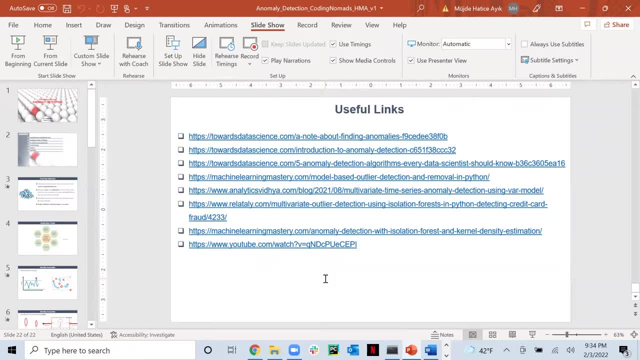 And we were sending this information back to Airline Operations Center And in that case that was basically to. the objective was to identify the faults before they actually happened so that I mean no accidents could happen or like maintenance costs could be solved and stuff like that. 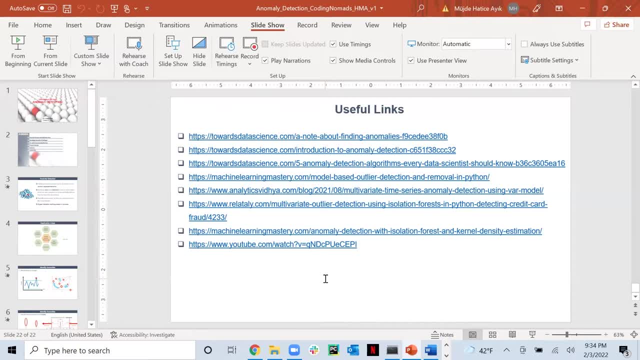 Or, for example, when I was doing for, like, missile flights, sometimes, when things are getting wrong and system health monitoring gives you some alerts, you need to take an action in real time, Even if not real time, because real time is risky, you can do this like offline and this basically helps the field experts that, OK, there's an anomaly here, so there might be some problem in this flight, although you see like everything seems OK. 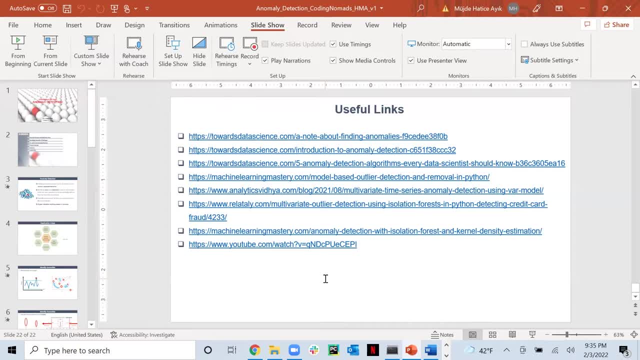 So basically we are identifying anomalies so that business can take action on that, Because anomalies are things generated So generally businesses want to take action, like in fraud, So in the, and that part makes sense conceptually. but for instance, could we take a look at the result of the isolation forest that you demonstrated? 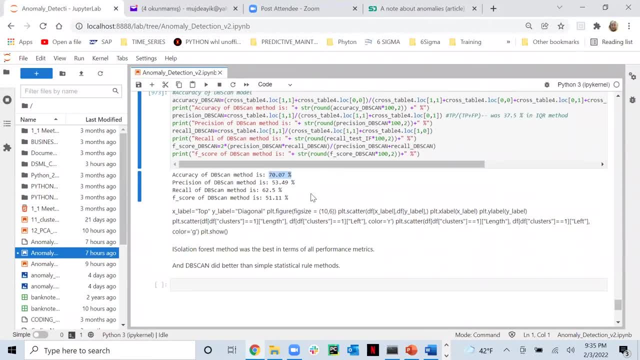 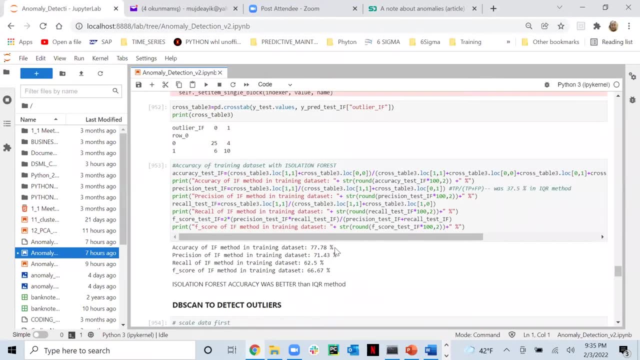 OK, So this is the DB scan, and just to use the best example, right, Mm-hmm, I think it was This one, This one. yeah, There we go, And so can you just explain this result to us kind of as simply as possible, if you don't mind. 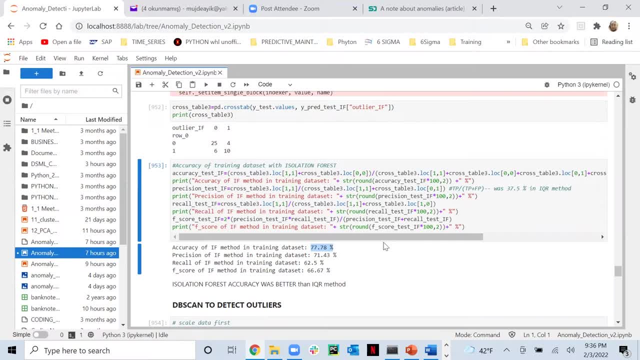 Like, for instance, up and top you've got the labels outlier AF01, and then for zero you've got 25 and four, and for one you've got six and 10.. Oh right, OK, Like. what does this mean? 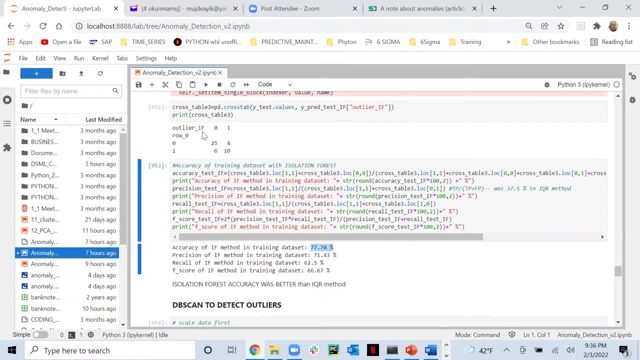 Like, what are we showing here? OK, So basically here what I am doing. Yes, So these are my outliers, So these are. so I have got like 29 genuine banknotes here, actual. 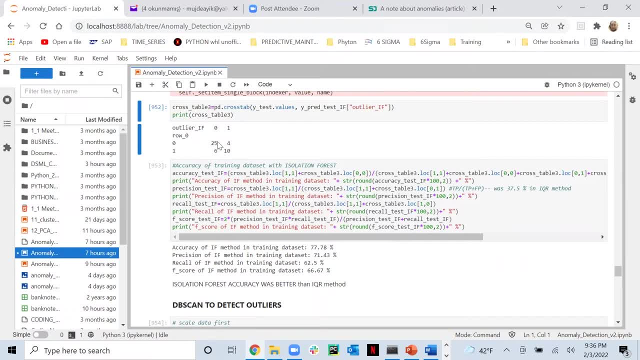 They are actually genuine And among those 25 genuine banknotes, So my model set 25 doesn't have any outliers, so they all look genuine too. So my model made a good prediction here. OK, But among those 29 of them, my model set, like four of them are actually anomaly, where they were not. 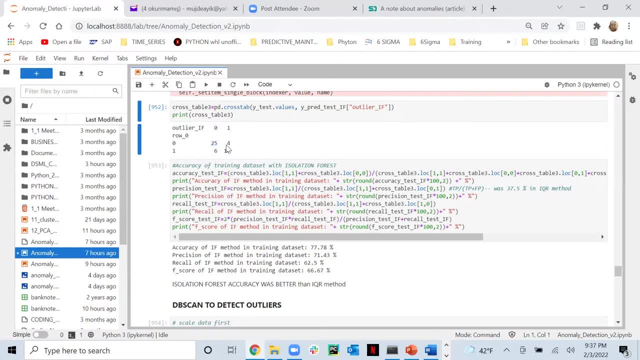 OK, And so this: obviously this is my sort of if this is zero, so this is my false positive Right, False positive, OK, OK, OK, OK, I'm really always confusing. I need to remind myself. 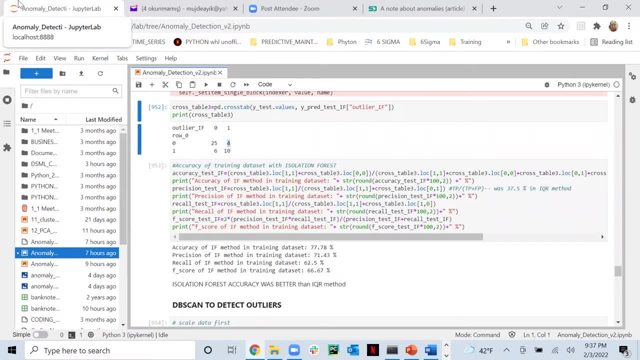 That's why it is called confusion matrix, Because they're so confusing. It always confuses me. But, for example, The most important thing I guess first for the students to grasp could be: you know, in the x-axis you are seeing the actuals. 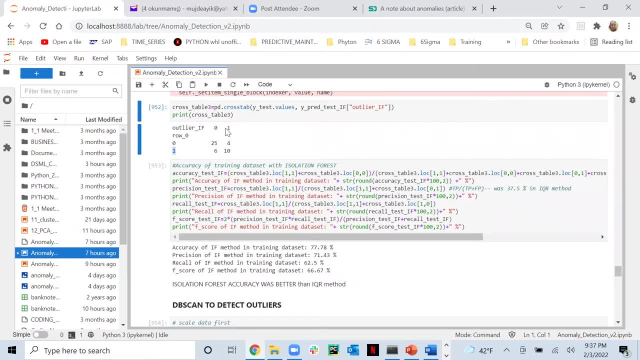 And in the y-axis you are seeing your predictions. Yes, Yes, Exactly So. in my actuals, like, for example, I have got 16 fake banknotes And among those 16 fake banknotes, I were able to identify 10 of them. 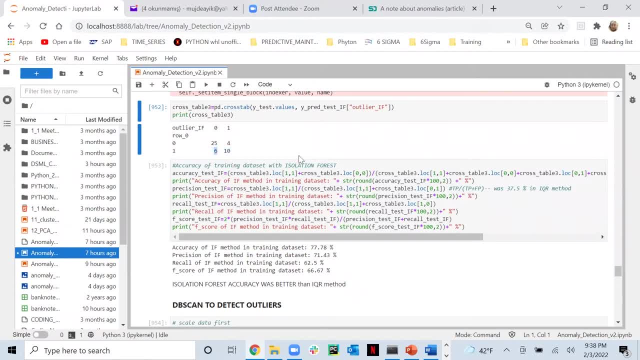 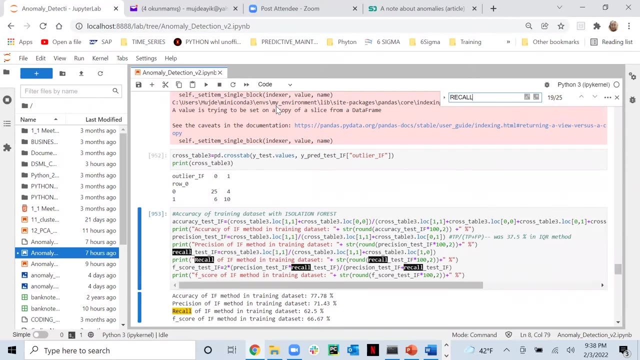 And I was not able to identify six of them. So this basically all affects my accuracy and recall. Actually, I reminded that to myself in some way because I know I will always get confused about these things. Yeah, those six cases are false, negative. 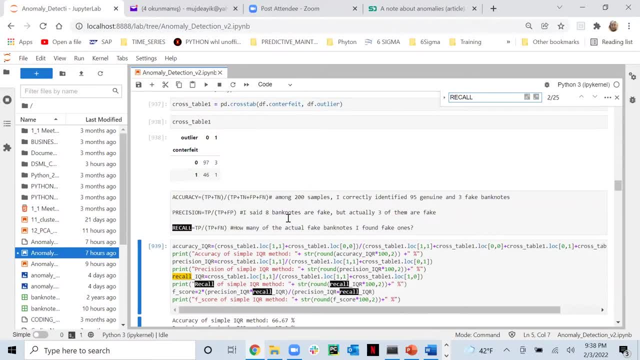 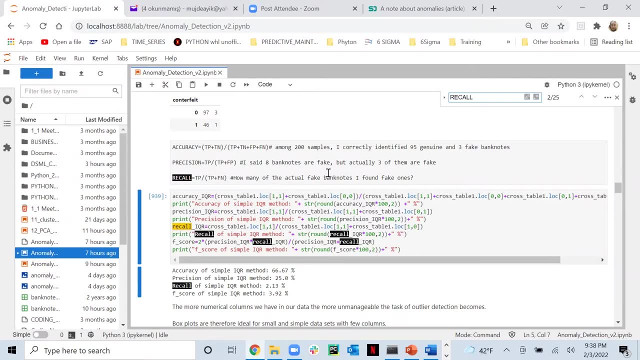 And they, They are more expensive, you know with cost, Because you were not able to detect. Yes, And because they are fake banknotes, it creates, you know, financial problems. Yes, False positives are like false fire alarms. 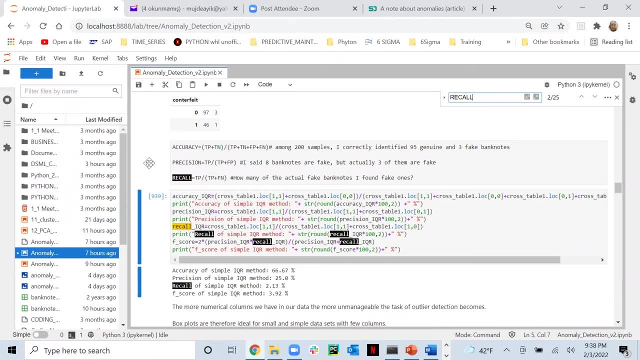 You just go out and come back. There is no big deal Like, for example, precision is here, like my true positive over true positive and false positive. So if I said like here, for example, an IQR method, 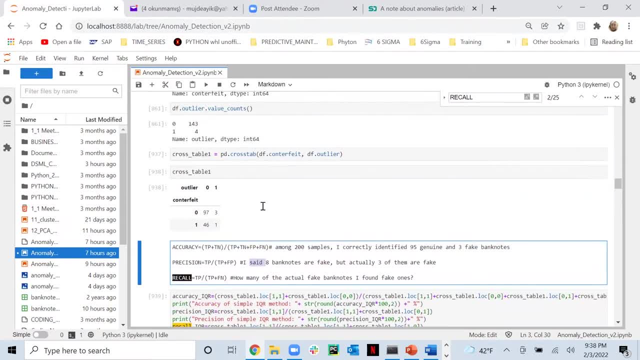 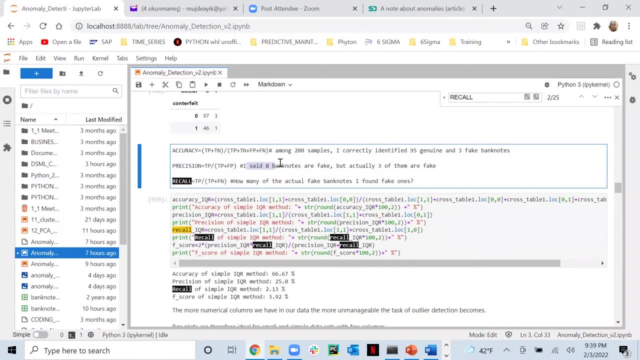 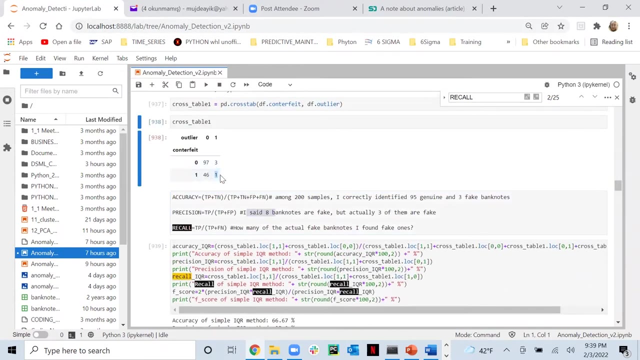 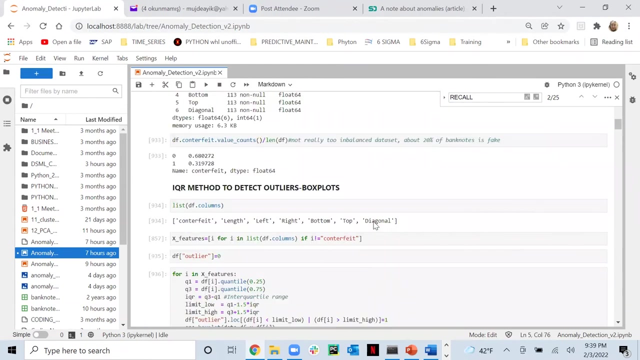 I think. So what is this? I said like I think I put a wrong one in here, But basically true, positive, which is here. Can I have a look at something? I think it's. I guess we were in the isolation. 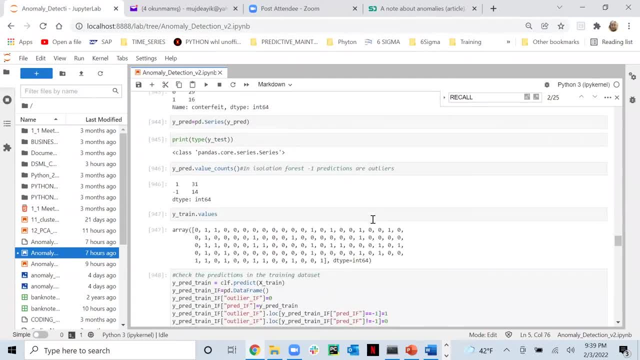 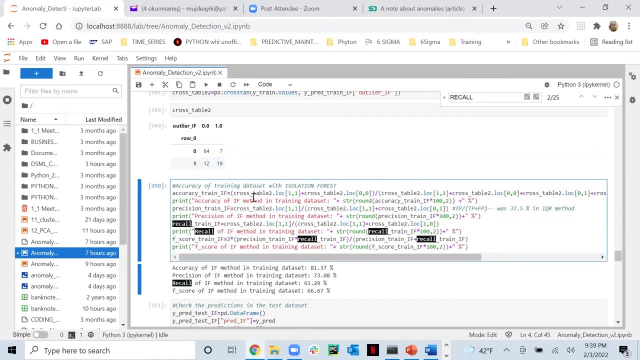 Isolation forest output, Was it? Yes, we were talking about the isolation forest confusion matrix. I mean yeah, So basically it's all about like accuracy is basically how well you are identifying the zero cases and one cases. 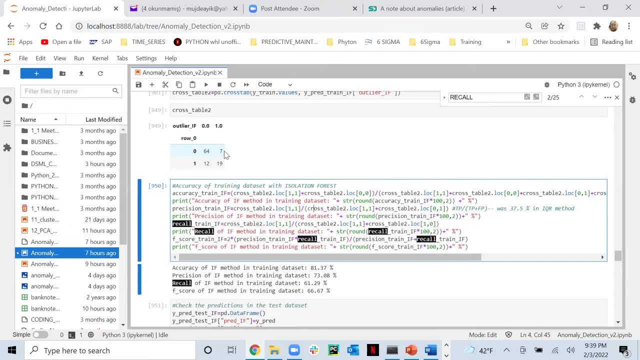 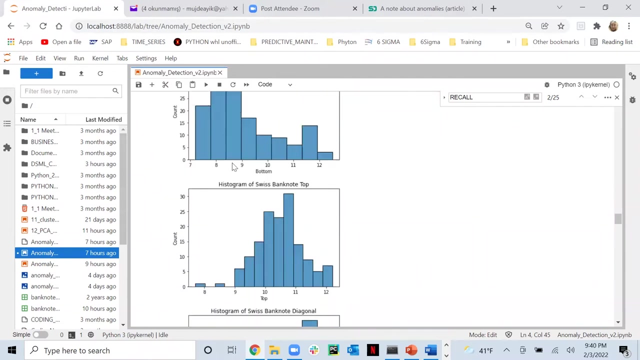 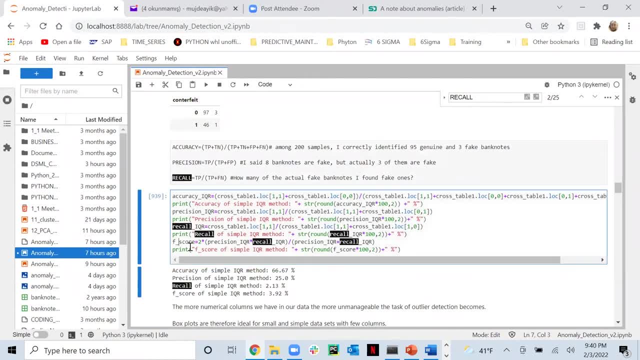 And once your data is imbalanced, basically, Basically, F-score is better to look at. I'm correct, right, Çağdaş? I'm getting confused. Yeah, sure, Of course This can. This is really, I guess, maybe a three-day course. 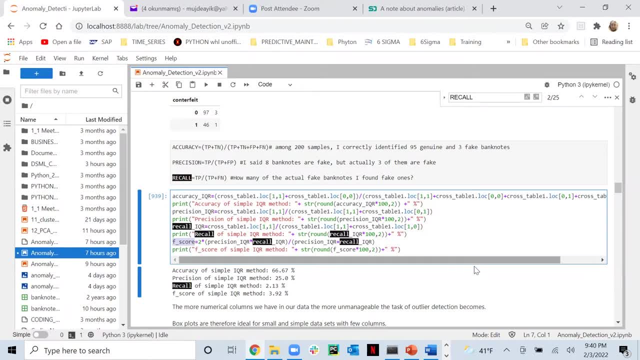 I mean the whole confusion matrix and maybe together with logistic regression and some anomaly detection. It can really take some time to digest And I I recommend to our students that you know they should really spend time on confusion matrix because it is a real common interview question. 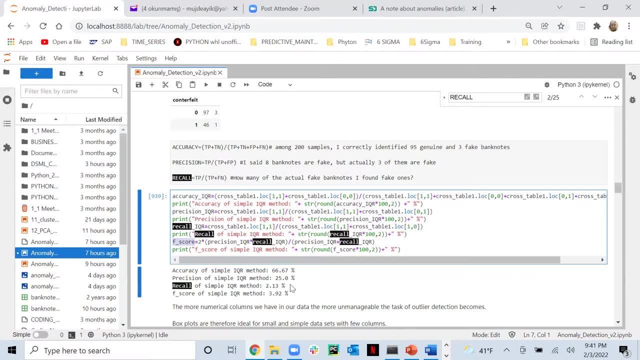 I can't imagine a data science interview without confusion. matrix, I get it again. I again forgot to name what I was talking about. Interviewers also get confused during the interview, which is also common. So can you, Çağdaş, if you don't mind, or? 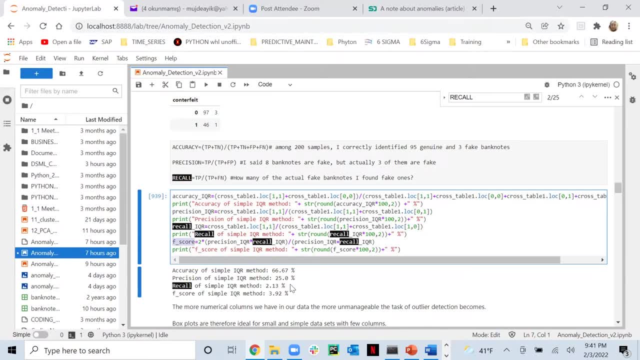 What is a what would be a good example of an interview style question, you know, related to the confusion matrix, Yeah. So, for instance, a question could be: imagine that you are doing classification, you have a classification problem and what would be your metric to understand? 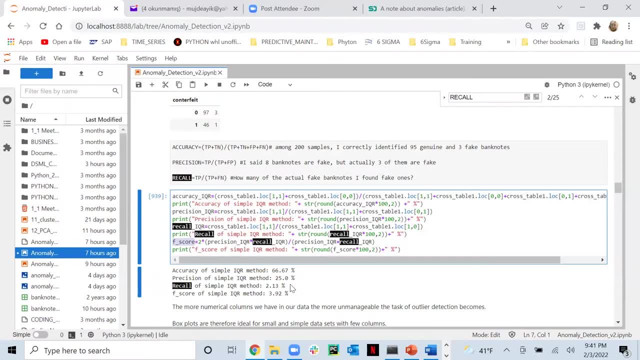 Maybe you have to understand your model's performance Or talk about your performance metrics when you are doing classification. So this is a common question And the answer is confusion matrix. I check my confusion matrix. I check my accuracy, recall and precision. 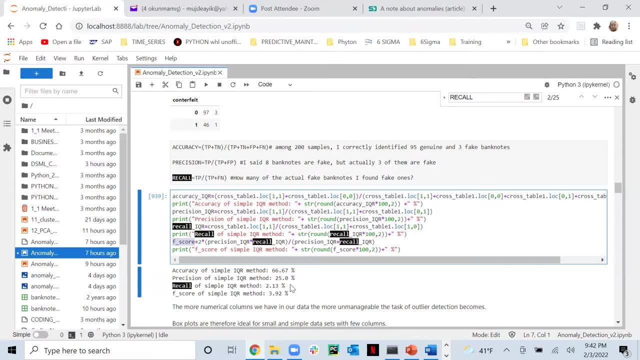 And F score is also a derivation of precision and recall. You just need to talk about the accuracy, recall and precision, And F score is also a derivation of precision and recall. talk about these metrics, It's a common question. yeah, I also, exactly-. 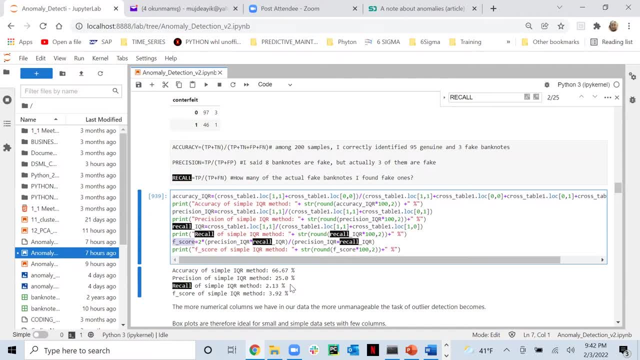 I can dig deeper. Yeah, like, for example, as you mentioned, I mean that question came to me and after that, just like in the course, as Gilad mentioned, then the interviewer asked me: like okay, you have got a, let's say, cancer data set. 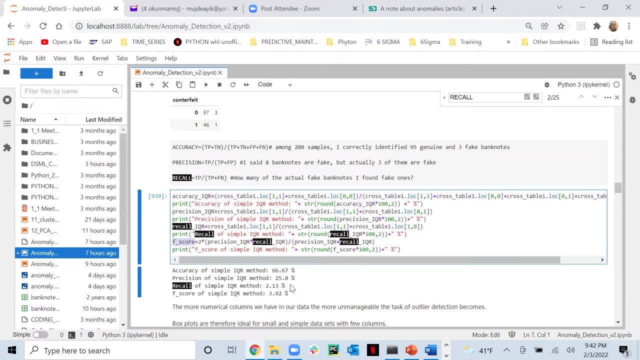 and only 10% of the data is labeled as one, So only 10% of people are cancer. So he asked: like in that case? in that case, like accuracy is a good metric to use, I said no because I learned from Gilad. 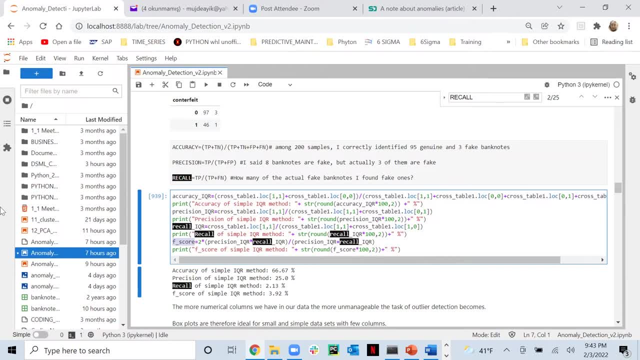 Yeah, it's so true. Yeah, it's true, because in that case, for example- okay, just like in here, for example- you get the- I mean, let's say only from from hundred data, you have got seven cancer people. 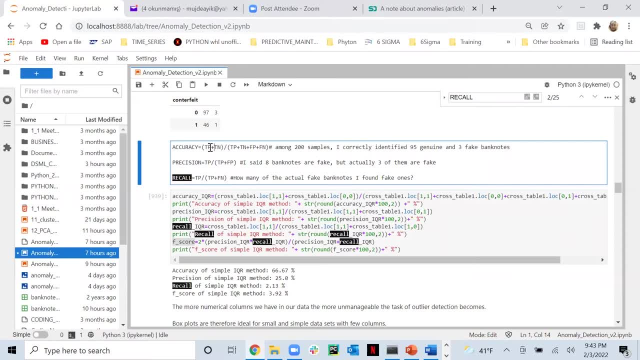 Even if you don't identify the cancer people right, you will still identify the non cancer people, right. But that's not enough for you to have a good model. Yes, a good model should perform better than the majority case If, in your data set, 98% of the data is okay. 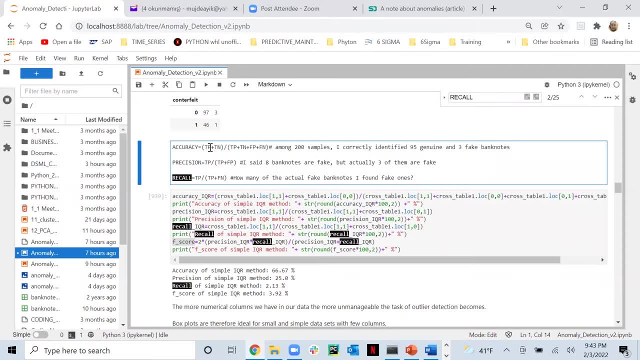 and you know 2%, you have 2% anomaly. Then you know you can just say all of them are okay and you are 98%, right, right, And you can claim that I have, yeah, 98% accuracy. 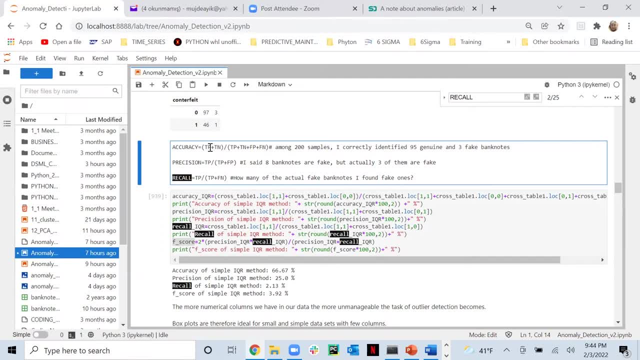 You are the king, but it's not the case. That is the question actually. That is a famous interview question they ask: You shouldn't be looking at the accuracy metric, You should be looking at the precision and recall metrics, And they are the ones in this confusion metric she just showed, identifying how precise the model is, capturing the actual cases and also how precise it is identifying you know when you predict anomaly, if it is really anomaly or not. 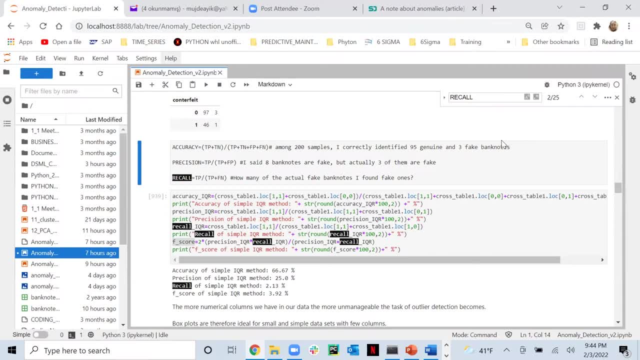 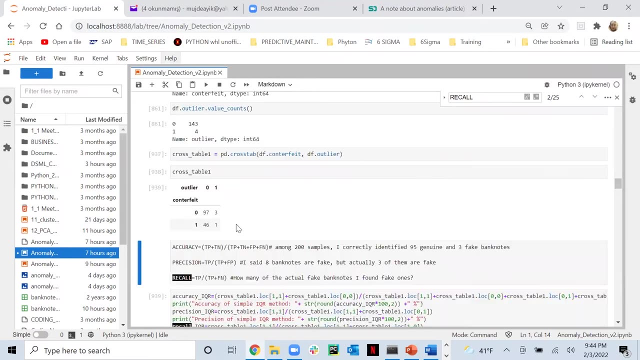 Maybe the last part of my sentence was also a bit confusing. but the more important things are capturing. you know how many cases you are capturing from the total anomalies? Yes, In, I think here I made a mistake. Let me have a look. 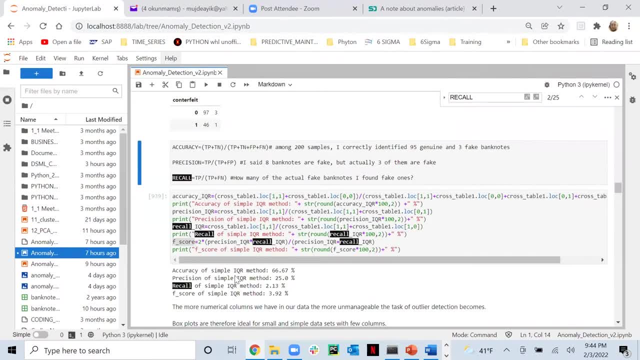 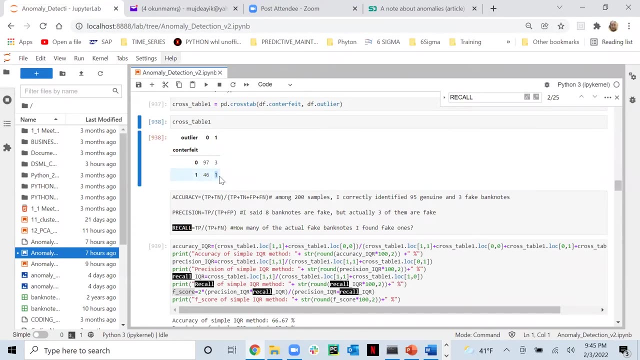 For example, here I said: what's my precision score? My precision score is actually 25%. What's my true positives? My true positives is this: right, Yeah, This model is capturing only one. Yes, So there are 48 anomalies in total in the data set. 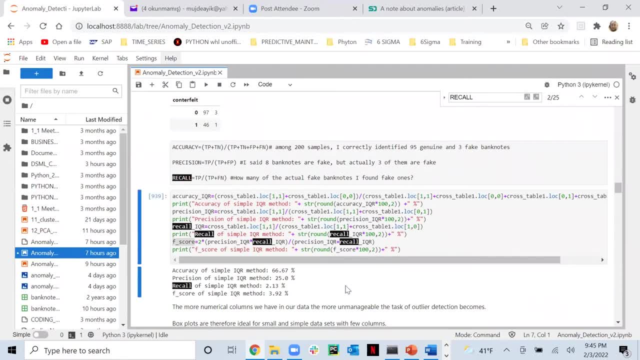 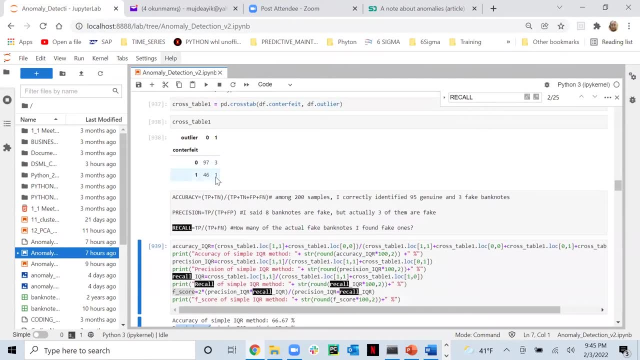 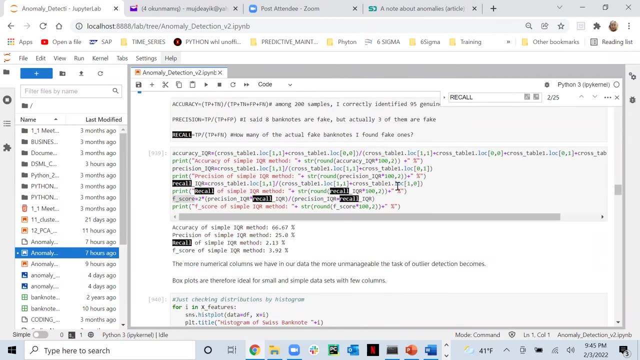 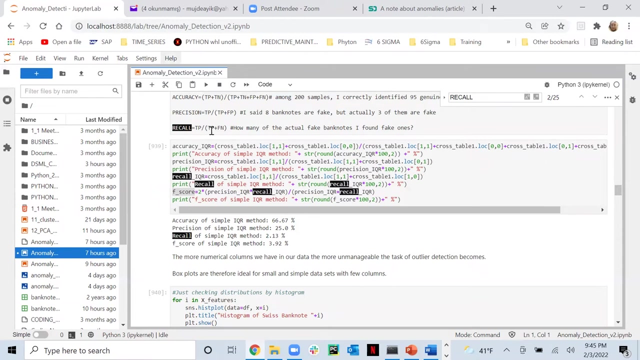 My precision is not good. So you see, like this is my IQR method and my precision is not good because it's only capturing one of the actual fake banknotes. Yes, And my precision So, but that data is imbalanced. or when you are not happy with those accuracy, precision stuff. 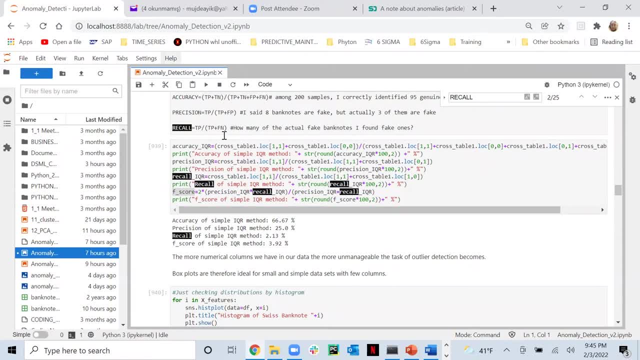 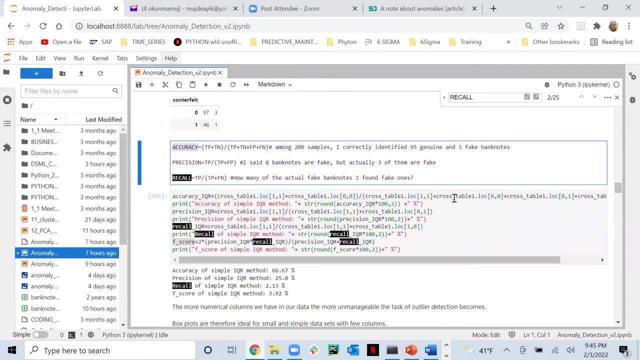 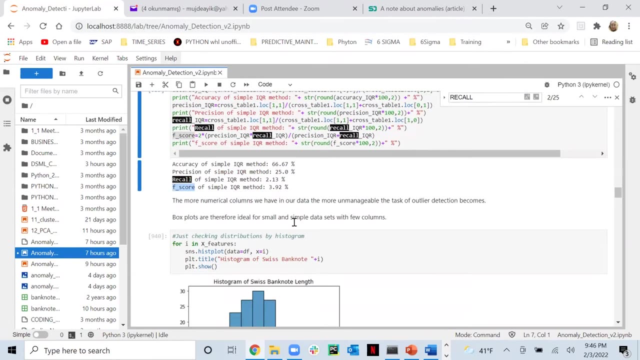 It's always good to look at the F-score, because F-score is sort of giving a balanced information on what precision and recall if accuracy is not appropriate metric for your problem, especially like in imbalanced data sets. So here we look like F-score is 3.92, which is really bad anyway. 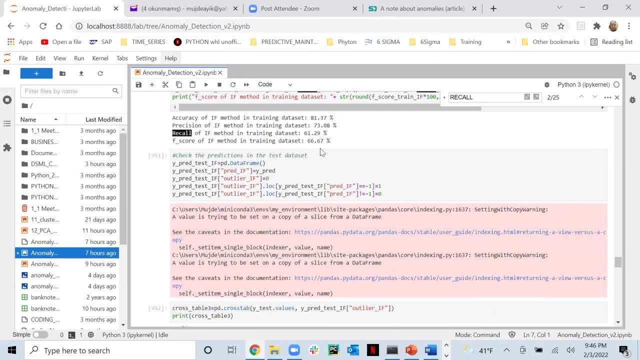 So if you go to like our isolation forest, for example, it gets much better. Yeah, that's the real improvement. You improve, Yes Score from three percents to 66 percent. Could you go a bit up to show us the matrix? 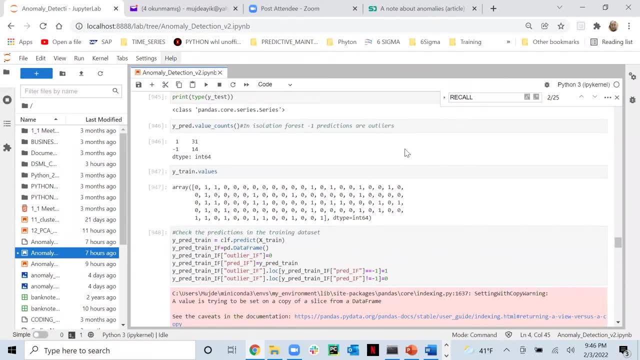 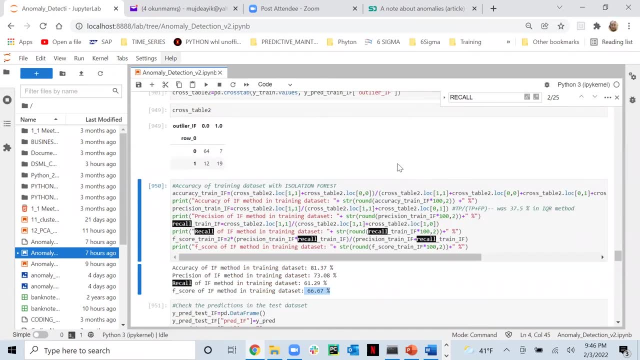 Okay, Stop, No, no, no, I mean the confusion matrix. Could you go down? Mm-hmm? Okay, Yeah, this one, This one is the matrix. So in here we are capturing 19 anomalies. Yes, 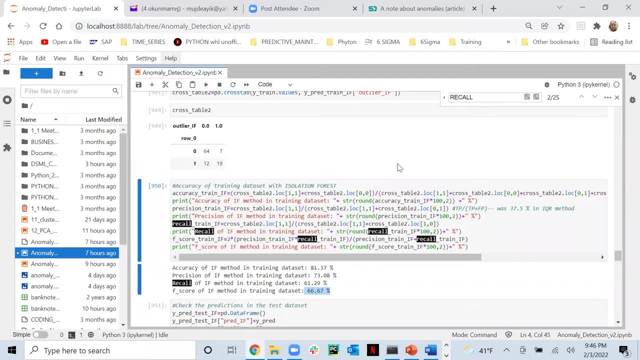 So we improved it from one case to 19 cases. Yeah, That's the, That's the metric we should be looking at. Yeah, And I think to take it back to kind of where my mind goes oftentimes with this, which is the kind of how this information could help a business decision right or in, let's say, a government decision- 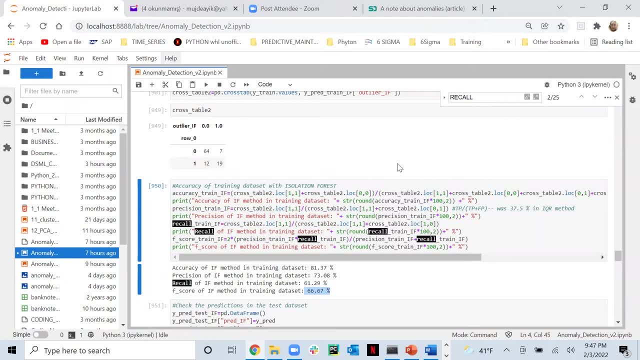 So let's say you've measured all, because the features of these banknotes are essentially the dimensions, right, and the physical attributes like the width and the length and maybe the weight, Yeah, Yeah. And so, given a sample of a million banknotes, when you analyze that data and you can come up with a, you know, 81% accuracy or 66% F score, there could be a spot where you say we can predict that the entire, you know, let's say, 100 million banknotes that are out there, this number of them are fraudulent or counterfeit or fake. 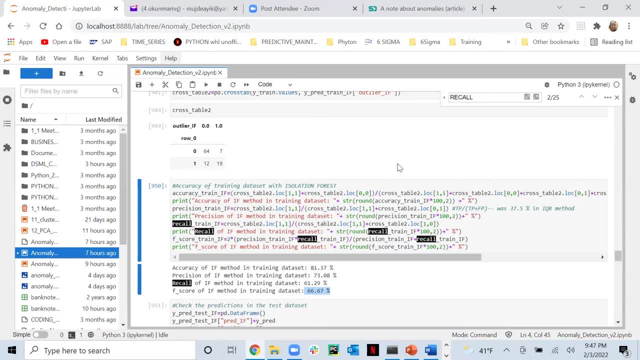 Mm-hmm, And at a certain threshold the government is going to be able to predict that. Yeah, Yeah, Yeah. And the government could then say, okay, we need to update, we need to release, like a new banknote or something. 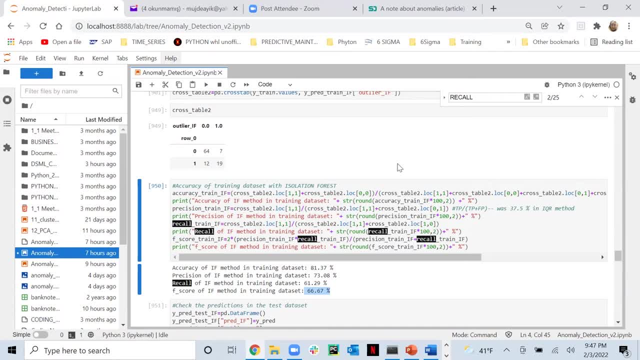 Mm-hmm, Is that about right? I mean it could be, because I'm not really a very finance person, I'm not sure like what action they could take, But obviously once I mean they would like to know about like fake banknotes or it could be the case like in, for example, exchange bureaus and stuff like that- they don't want to get like fake banknotes. 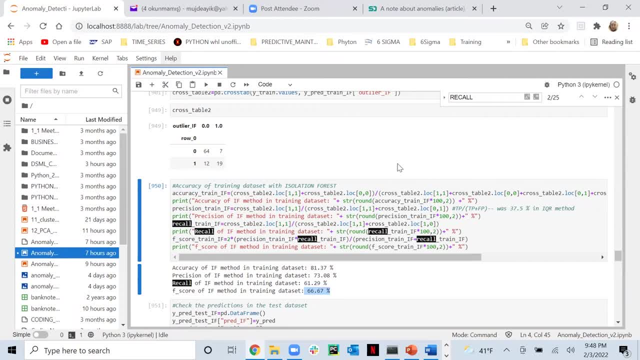 And there should be some action to take when there is some anomaly. I think business in that respect would know that better. Maybe each other you can say: but it's a business decision And that just sounds logical what Ryan just said. 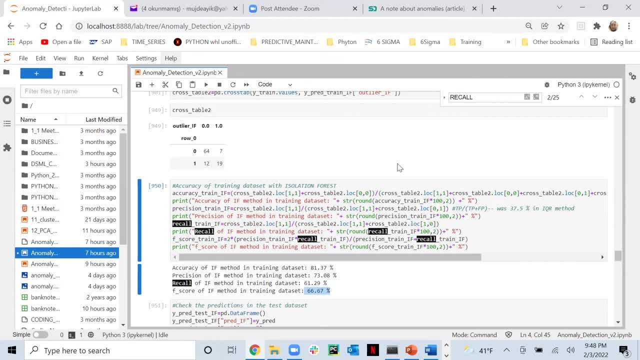 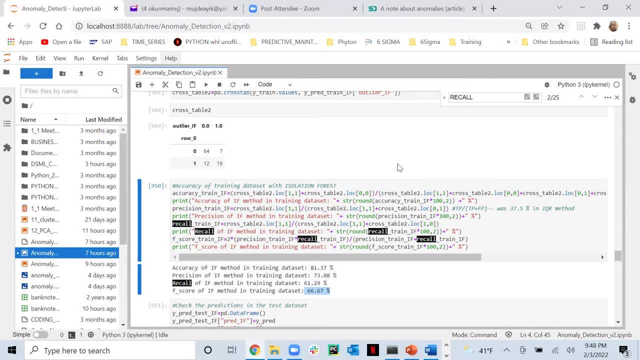 Or credit risk scoring for individuals, for persons for banking in banking industry. would you give someone credit or not And you maybe identify some persons, some strange transactions using some of these methods? Yeah, I mean so. Yeah, Yeah. 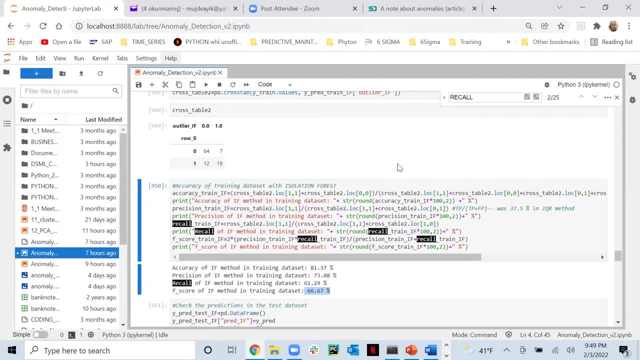 Yeah, insurance field they were trying to get this anomaly, anomaly behavior so that they would sort of trying to capture fake claims. So in that respect, like they wouldn't renew their policies or they wouldn't get that kind of customers just at the from the beginning when they apply for a product, 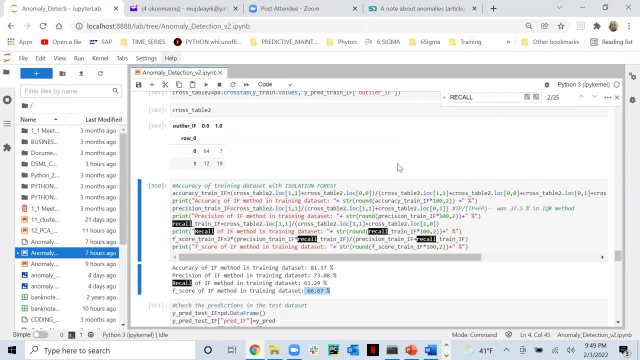 So those kinds of actions the business can take. And then in the, in the case of fraud detection right at a bank, let's say that we- and it's unsupervised, or you know, we're basically looking for real fraud, the cases of potential. 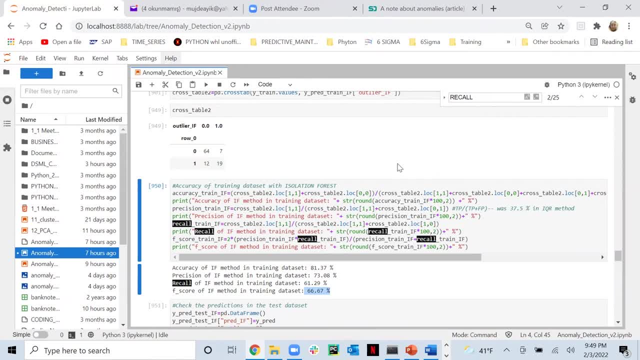 fraud and, let's say, transactions, And we want to then actually go, you know, forward this outlier. How do we, based on from where we, from where we are here, how do we get back to the end, the actual data point that that we have detected as an anomaly? 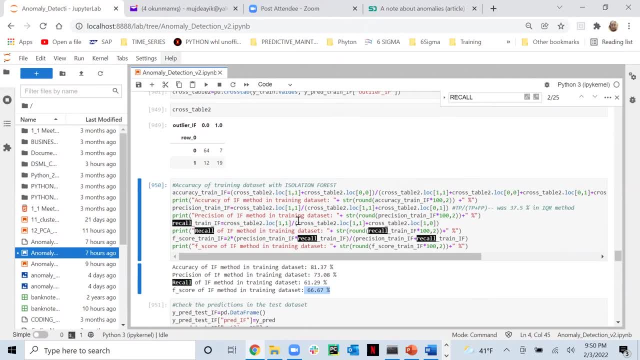 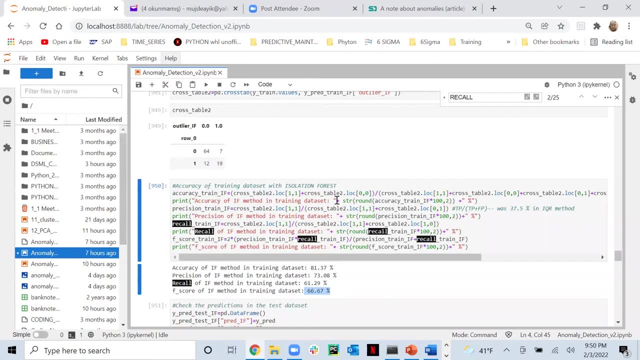 Actual data point I mean in this code, So we can think about visa or MasterCard transactions live streaming globally. huge operation right All of a sudden, from your credit card a huge amount was seen, you know, in your purchasing. 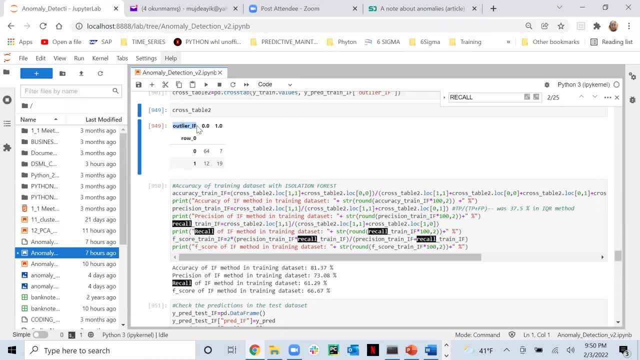 history there is no such number. Actually, this is a simple model, But just to give an example. and then the action is immediately to block your credit card from the bank- And this actually happened to my wife- or notify the customer somehow. I mean yeah, 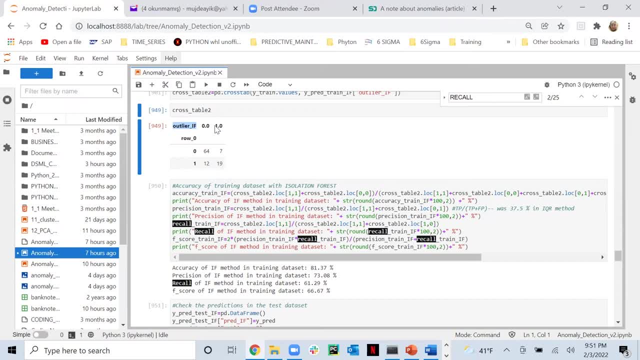 That's what I meant by fraud detection. My experience was, as I said before, with robots, sensors. Yeah, So you have to get the data And in that case, when the model, the tax anomaly in the signal, there were those signal. 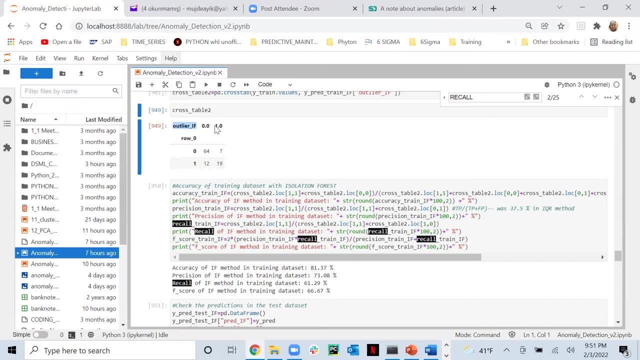 curves, like she showed, And the factory floor employees. they immediately stop and reset up the machine because the curve starts changing And it affects the car production. So that's another example can give. sometimes it's like an early indication of a fault. so before a disaster, accident would. 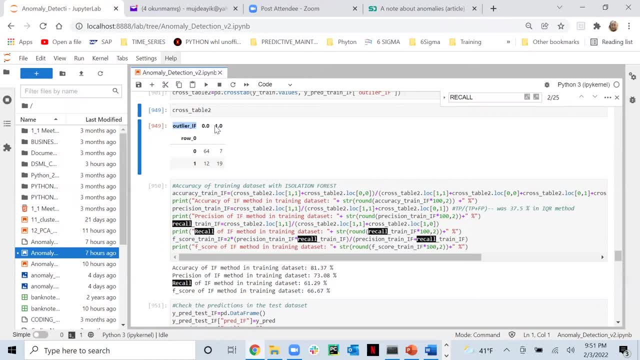 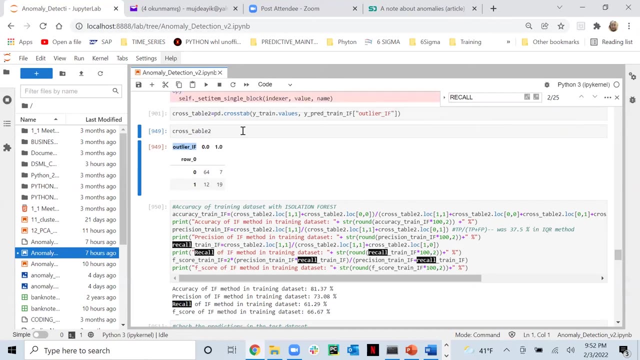 happen, you early detect it and you get the vehicle into the maintenance kind of thing. so it's an early detection of, um, some uh drastic event really. so a little bit if you scroll up just a little bit, and my apologies if these questions are uh too simple, but essentially, 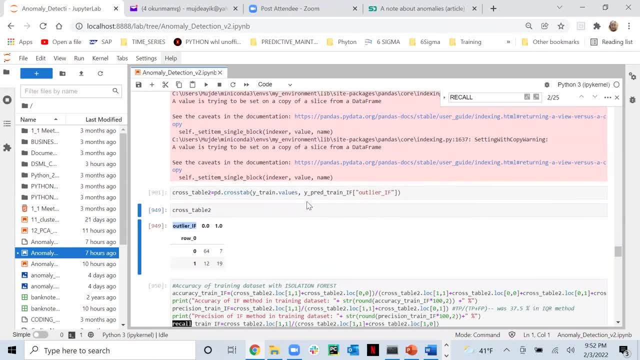 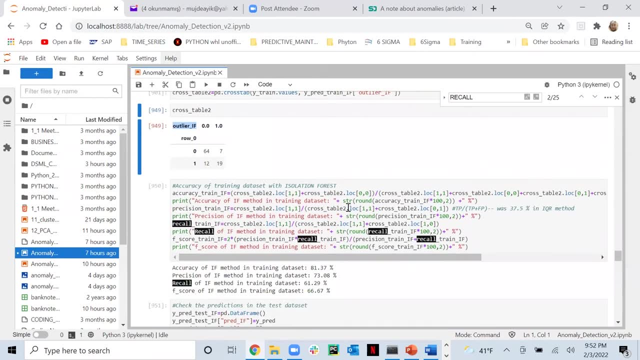 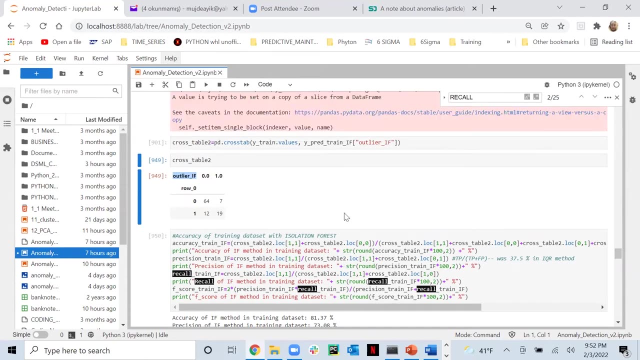 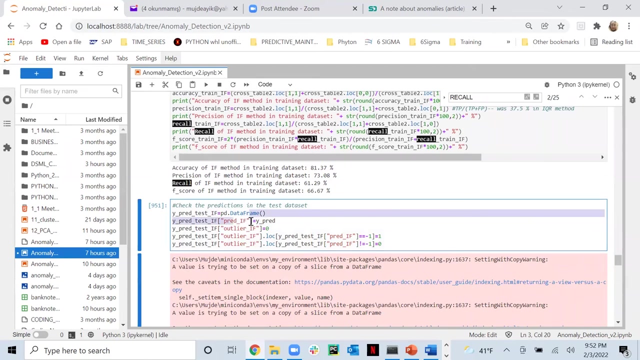 in in the code when you detect the anomaly. essentially, at that point you could then, um, you know, write to a file or raise a flag or, you know, do whatever you need to do programmatically to to address this potential anomaly. um, yes, got it. yes, yeah, basically, when i uh find an anomaly according to my model predictions, i just label, i just add. 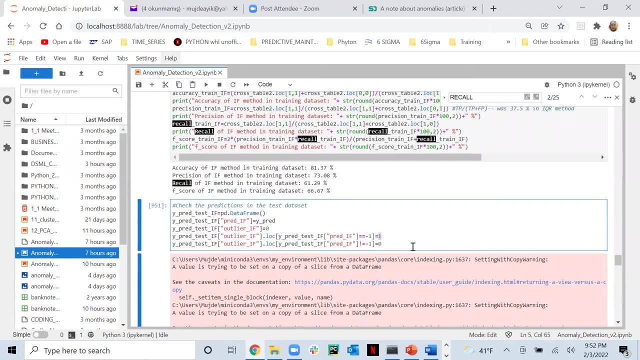 another column and label it as one, and later on i can just call it back. so i know which data points are anomaly and i can get them back. i can load them. got it, got it, yeah, nice. so, um, scott had posted up something, uh, where he was saying he doesn't have a good enough understanding. 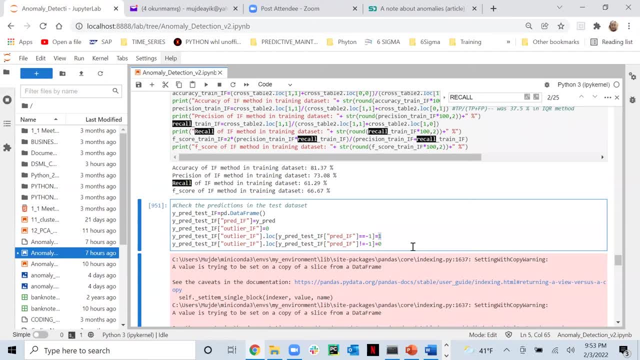 of these type of topics? that's an interesting question, scott, i'm with you a hundred percent. i feel like i'm drinking from the fire hose here. i know, i know just enough to almost follow along with all this stuff. um and uh. so, yeah, this is a very uh um. you know, this is, this, is it's kind of a. 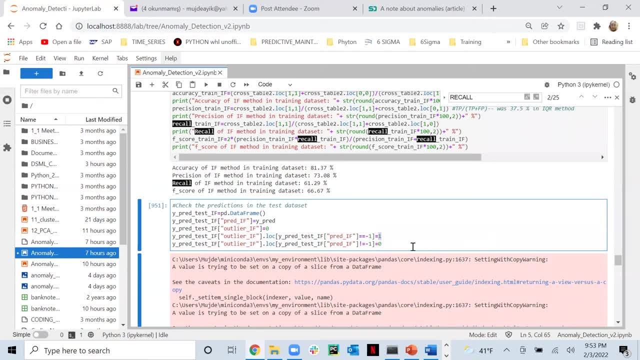 deep dive on the topic. um, you know with, uh, you know, obviously, you know mushy, you're an expert, shadash you're an expert. so you guys just listen to you guys talk. i'm actually getting a lot more. you know, uh, often, if i listen to, you guys go back and forth and and some of the questions that are 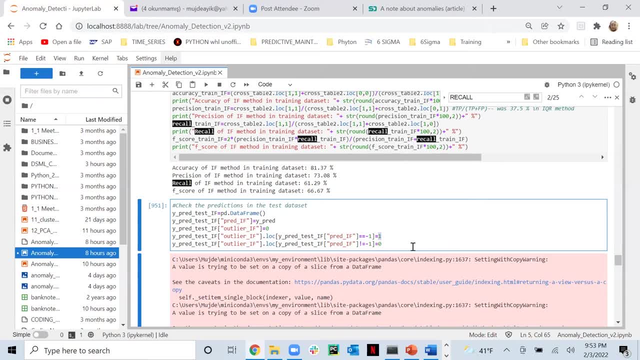 here. so, um, but one of the things that he says, and and again i'm going to parrot it here too- he says: it's it's fascinating to see the variety of libraries and techniques that are used to analyze data and produce results. uh, you know, going from some abstract glob of data to telling us something. 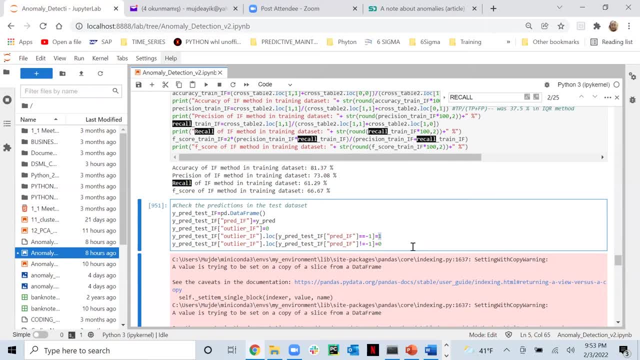 useful or enlightening, uh, which is, you know, not going to be obvious without all this analysis that goes on, and so, um, you know, for, for folks who are seeing this afterwards, um, who are watching the youtube video and looking at this, going, what the heck is this all about? can i go with it? this is, this is um. 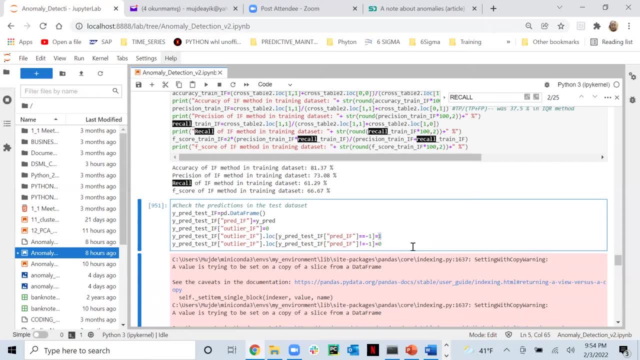 this is all good stuff and you know, um, i don't need to understand it all right now. i can, um, you know, i may pick up something later and then all of a sudden i'm going to connect it back to what was talked about here. um, so, um, you know, this is all interesting stuff. i've done very 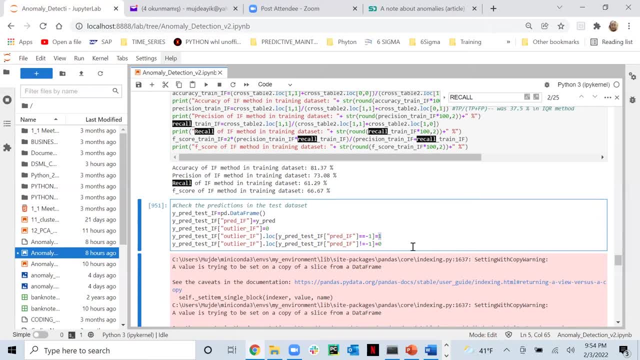 much in the way of data analysis and certainly nothing to this depth. so this is, um, you know, very interesting and very, you know, very good to see all this, all this stuff here, especially for me, the big thing here is just the, um, you know, the use of the, um, uh, use of the jupiter notebook to do all this. 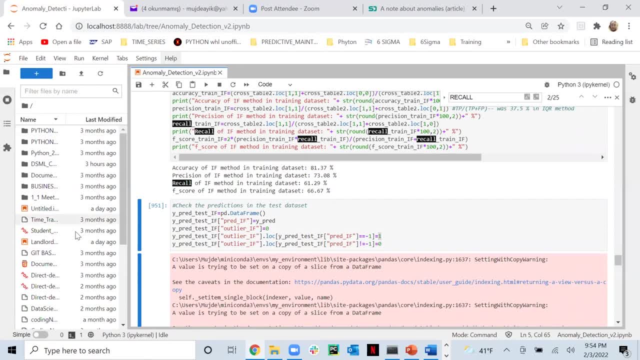 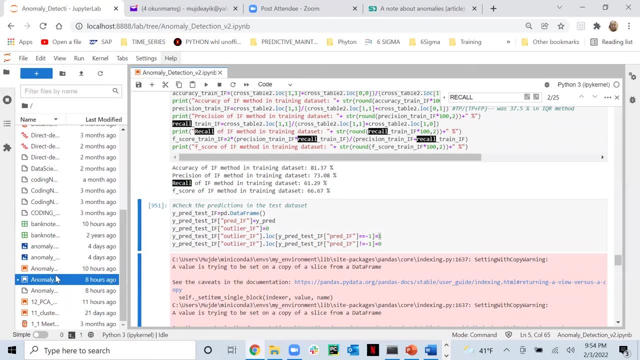 analysis and just come up with all this stuff. so that's always lots of fun. yeah, actually i had a photo as well. i would like to show that as well, but i mean maybe, um, because i'm not familiar with the moment. maybe, uh, am i? was i too much into detail? i don't know how the content should be. is it should? 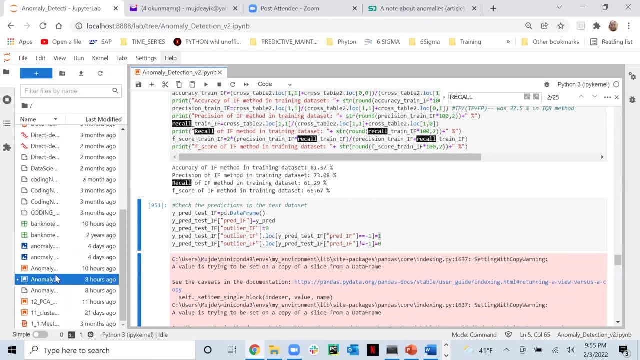 be like: uh, you've done a fantastic job, i'd rather have too much, i'd rather have too much information than not enough. yeah, i can't, i really um, even myself when i was explaining each other also, you see, like i'm getting confused myself with those metrics and stuff. i mean, they really need some. 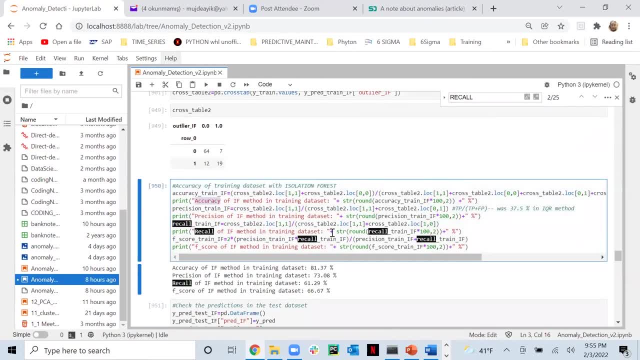 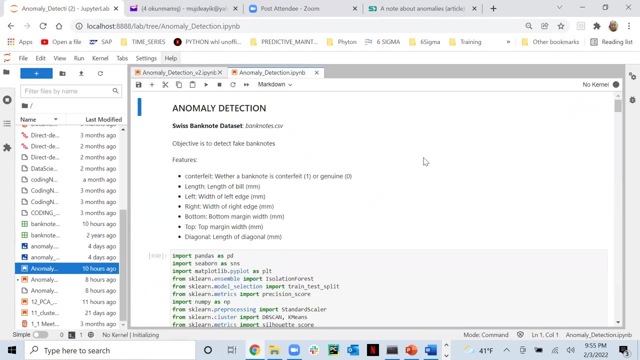 uh, but i think especially this accuracy. but elath explained in the course very well, there is something nice about these notebooks that i like. uh, you can schedule them. you can write a clean notebook and you can schedule it to run every monday evening, for instance, and then it can write. 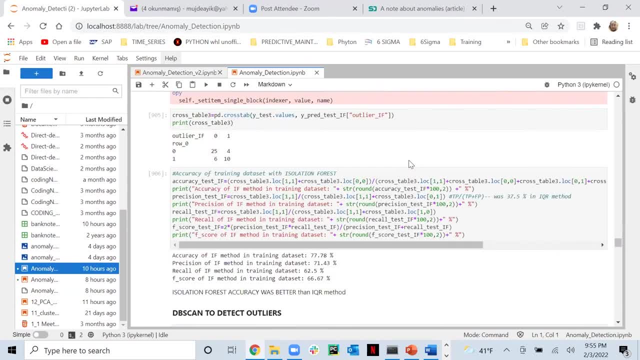 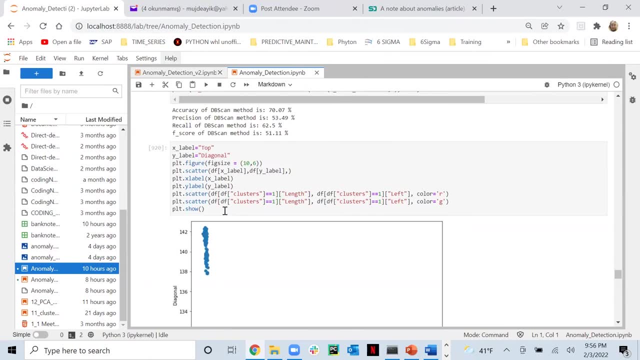 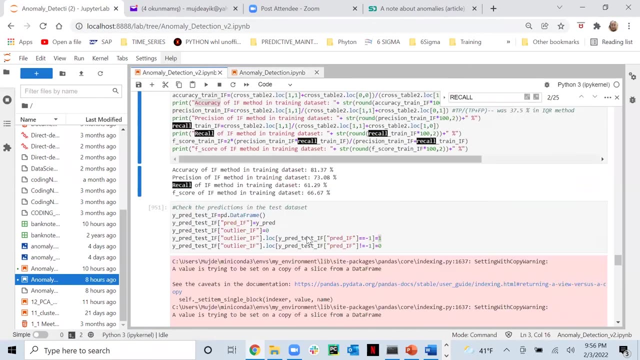 the output csv file to a folder where a data engineer can read it and use it in wherever they want. it can send it to a web server where you have a web application. it can look uh different, but notebooks can do that, yeah, yeah. so, and now you can just automatically basically: 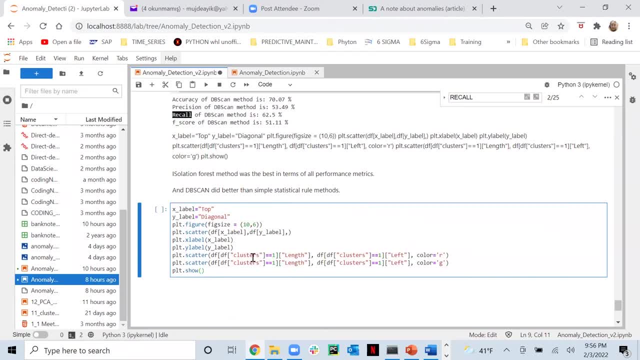 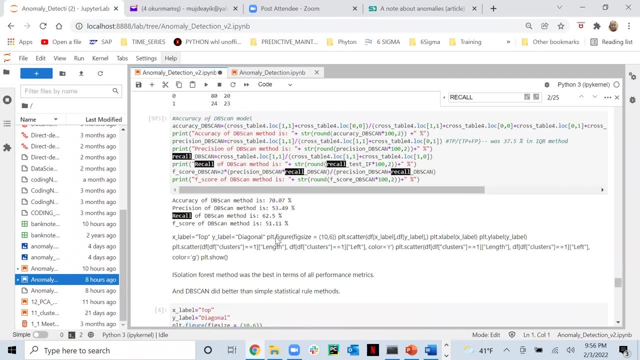 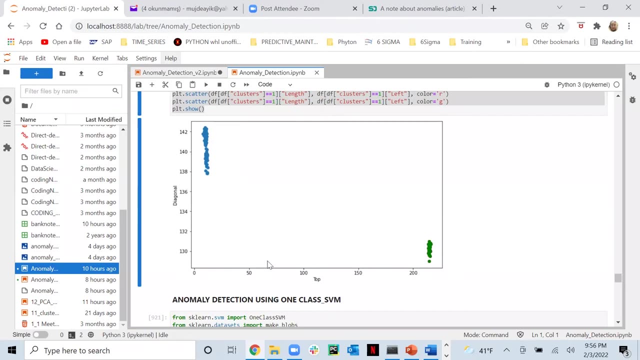 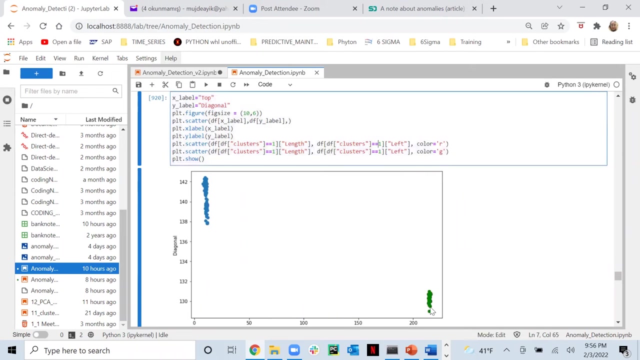 report. um, i'm just going to try something anyway. i mean, you can also like: plot all this stuff and, um, maybe in terms of different features, uh, i basically tried to hear here like: uh, try to plot the anomalies which are basically here on top of my predictions, and they are. 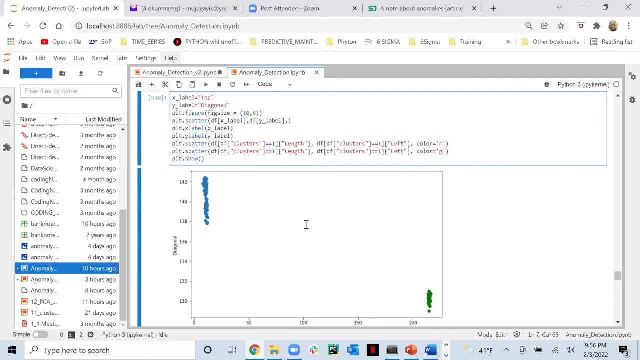 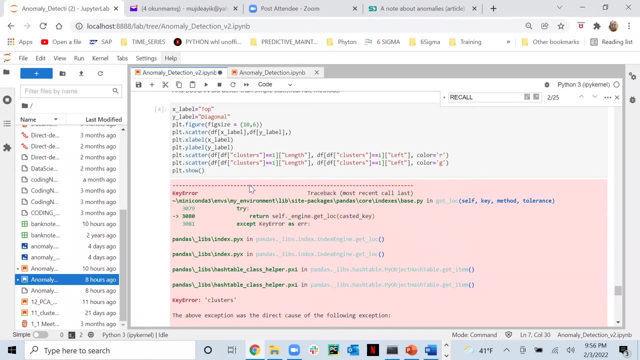 they were mostly on top of each other, but uh, anyway, it's difficult to show it here now because i got an error and there are sorts of things that you can do to visualize and to report to results to business. obviously, this would not be something to report to business direct. instead, we'll just 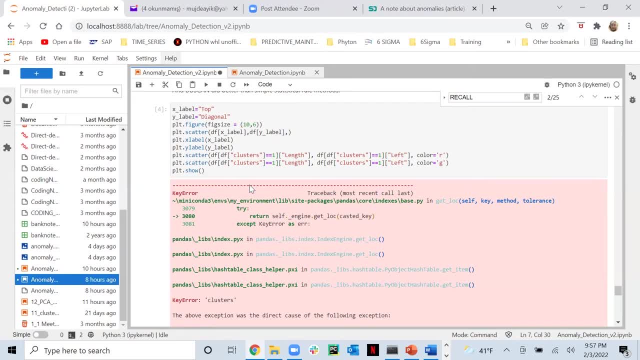 show some, some charts. you would just mention about your accuracies and precisions, but in a day they could understand. i mean, this is like, um, really at a tech talk it's uh, not a very much into business representation, really right for somebody then. oh yeah, i was just curious because my, that's, that's, that's the question. 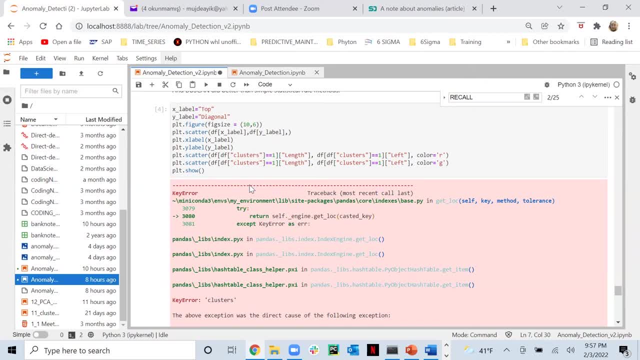 i always have oh, um in my mind. i'm always when, when we talk about the models and topics, just like this, i'm always thinking, okay, with this, you know what, uh, and i'm trying to wrap my head around kind of what can happen next, right, and which helps it make sense in my head? uh, but this has been this. 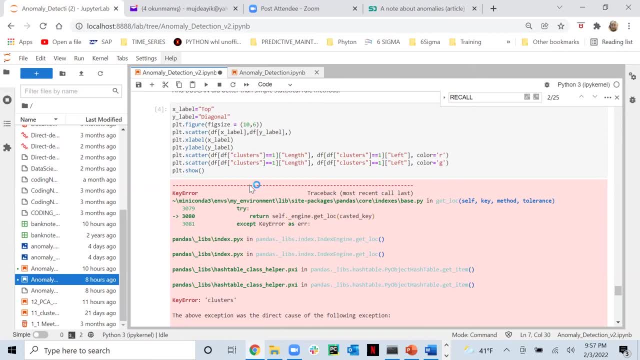 but, um, so i start to have, uh, a lot of questions and i'm kind of, you know, i'm i'm with john and scott and that most of this is flying right over my head. but i'm kind of following along and thinking and seeing how, how interesting it is and it really honestly makes me want to dive further into it, and 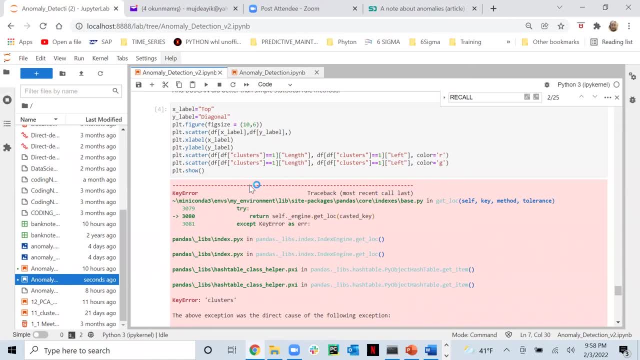 uh, and you know, basically, for the person that's really interested in this and uh, it's flying over their head both, uh, muzha and shadows, what, what is? what would you recommend as good next steps for that person who's just watched this, is really interested, doesn't fully understand what's happening. 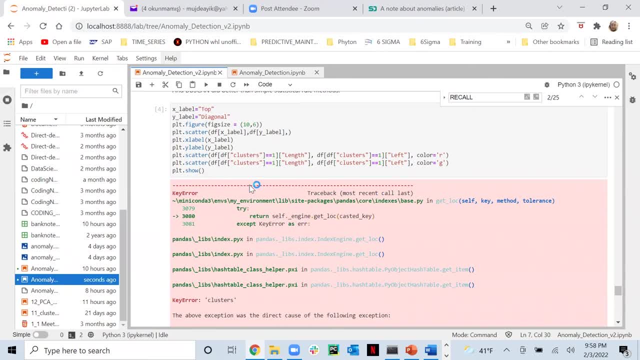 happening here but wants to be able to like what? what are some good next steps for them to take? uh, just, let's say the person already knows python. yeah, get in touch with us. that's a great. i mean i have also like given lots of resources, but uh, i know where to take. i mean, just by the 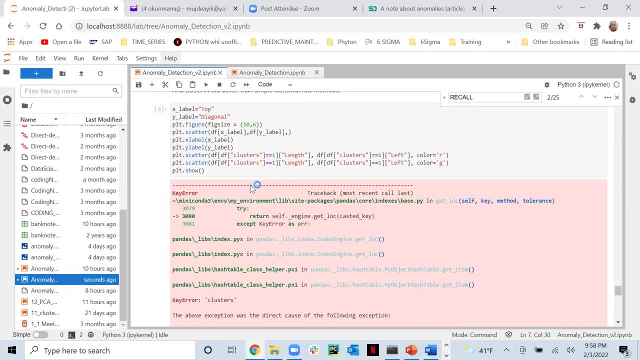 name suggest. i think in general this could be thing like: anomaly is something that we don't want, anomaly is something that is not expected and when the business and business doesn't like unexpected things and business wants to sort of alert beforehand, uh, the uh anomaly happens, uh and they want to take action and because they can't really do this, uh visually all the time and 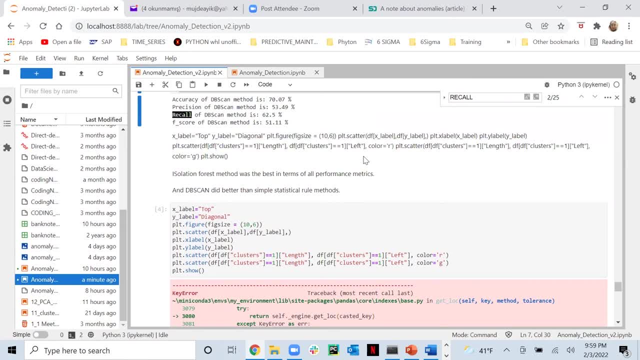 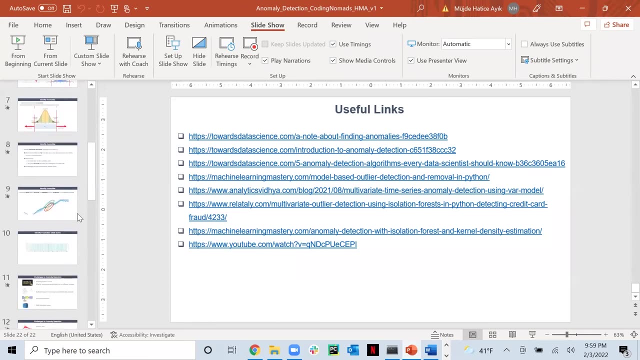 in time and all in this feature dimension space. we need to find a way to report them. hey, this looks like an anomaly. you may have a look and take an action, uh, kind of thing, uh, but i mean, uh, you, if they are into that, there are really many, many resources and there are many, many methods. 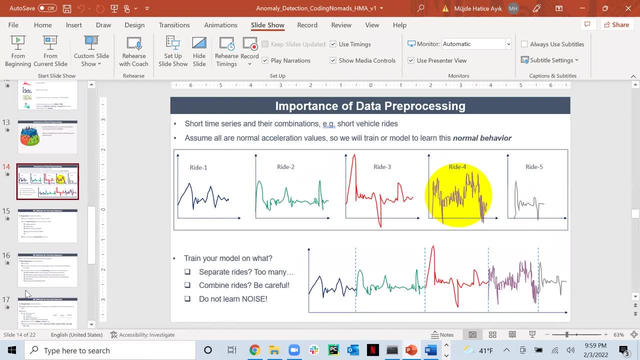 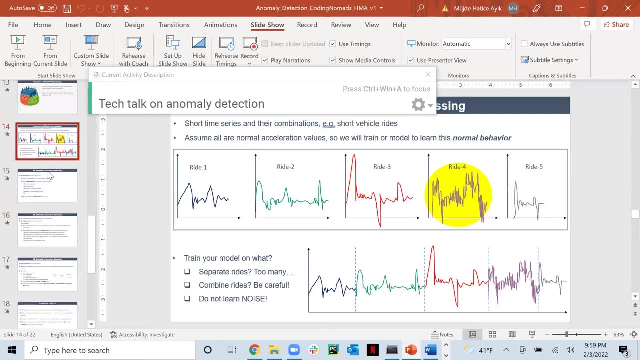 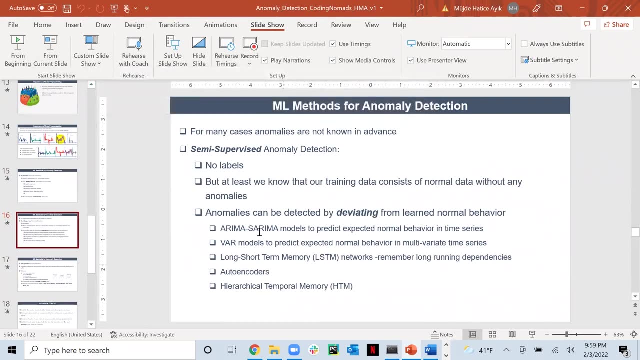 uh, they can just start with like one of the um, i mean i don't one of them. to start with those techniques, where are they? machine learning techniques, um, there are many. i mean they could, if they are interested, more into um, those uh like time series problems. these are the ones to go ahead. 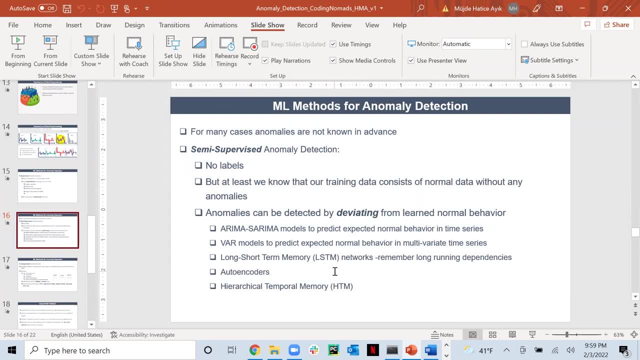 i mean they can do like time series, anomaly detection. they can just uh read articles and stuff like that. i mean there are lots of things on the web so, uh, they can always get in touch, i don't know, uh, yeah, yeah, the next step, the next step would be, uh, getting really comfortable with the central limit theorem. 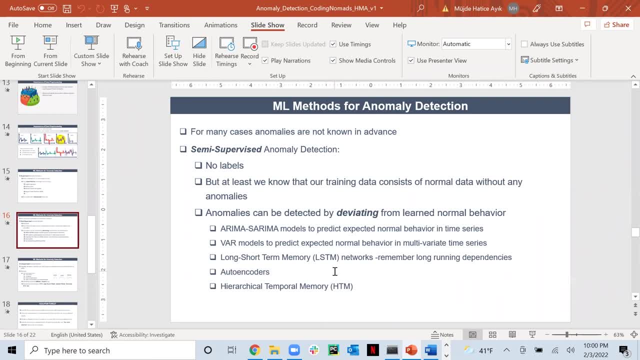 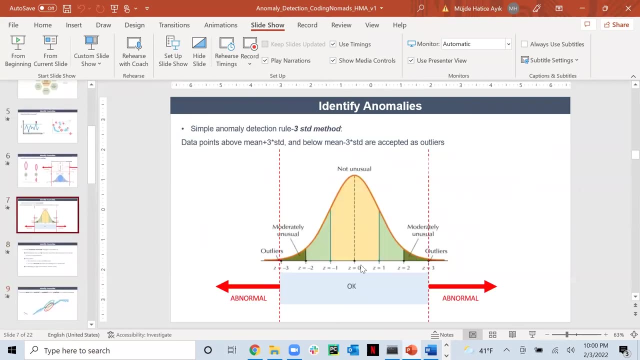 basic statistics, um how to understand the standard normal curve and how to identify, um differences in your data in using basic statistics. so that is the key, uh, i guess, to 80 of the problems out there. yeah, this one. so this can really solve a lot of problems. 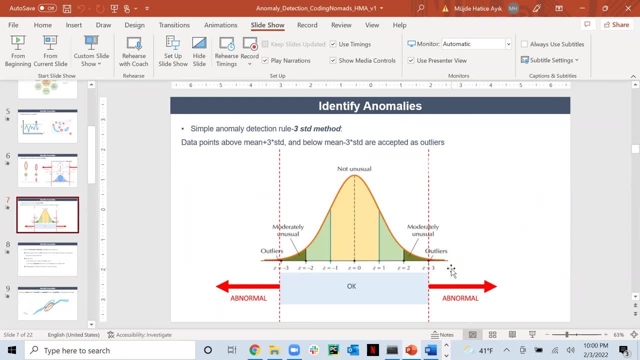 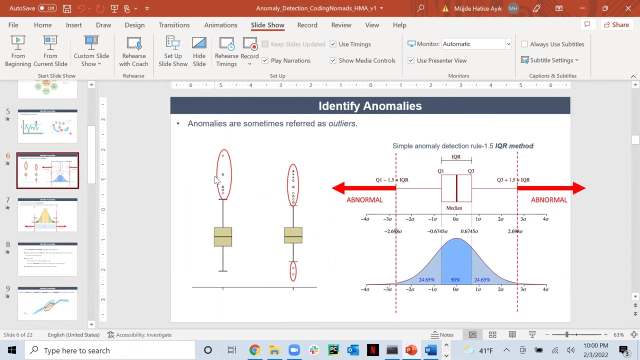 um, this is, this can be a next step for the students to also um, also, i mean, sometimes the objective is not really anomaly detection, But sometimes we are just building up a different model for different purpose. But even in that case, I mean outlier detection is something we- I mean we- have been looking into in our data exploration stage. 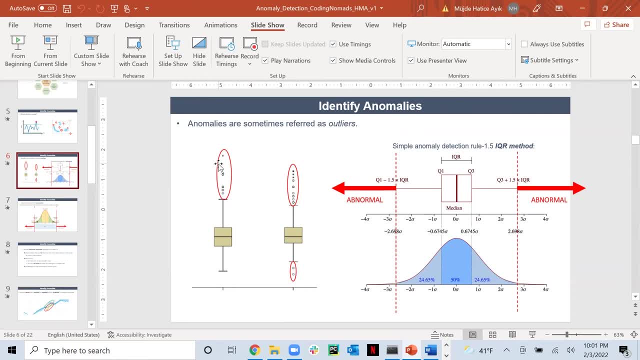 And because they could distort our- I mean- models and what our models is learning, And they are generally rare events. We always try to find a way to deal with those outliers. If they are not too much, we get rid of them, If they are not too much. 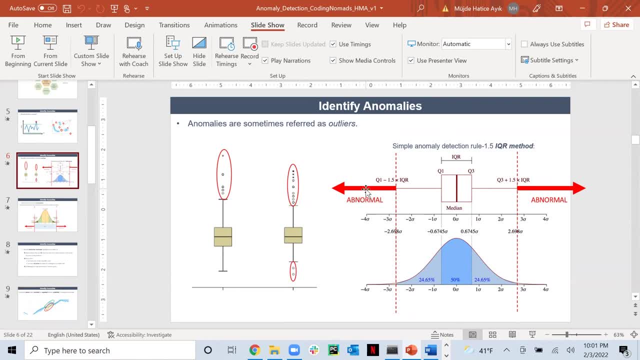 Sometimes- I mean again, field expertise is very important here. Sometimes we get together with field experts and they say, OK, are they here? OK, get them back to here. I mean, just shift those values sometimes. But sometimes we are just trying to find a way to deal with those outliers. 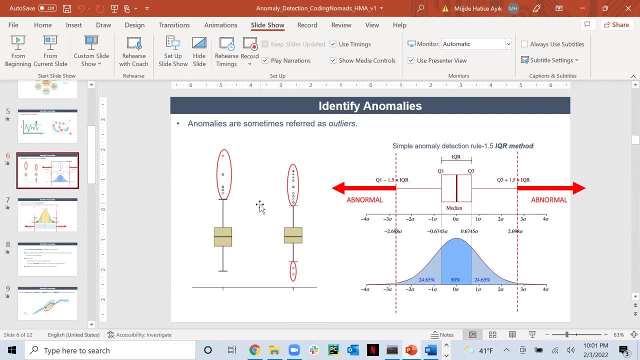 But I mean just like missing values, outliers. dealing with outliers is another stage in data preparation process. Even if your basically objective is not to identify them but just any other model, they may be distorting your results. because I know we're over time, I have one more quick question. I actually have to run really shortly too. 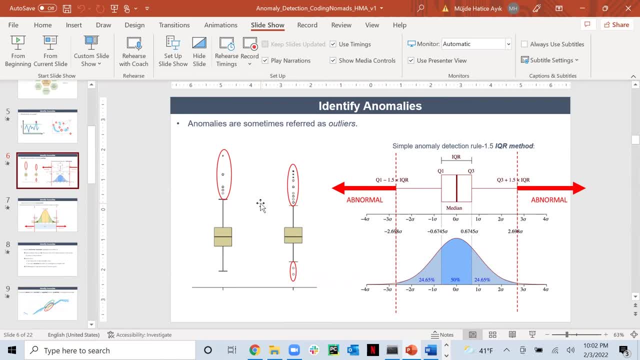 You mentioned data preprocessing. Are there common techniques for is that kind of on an ad hoc basis, based on the data set and based on the requirements and the noise in the data, Or are there custom- not custom, but regular- tools that you're using regularly for data preprocessing? 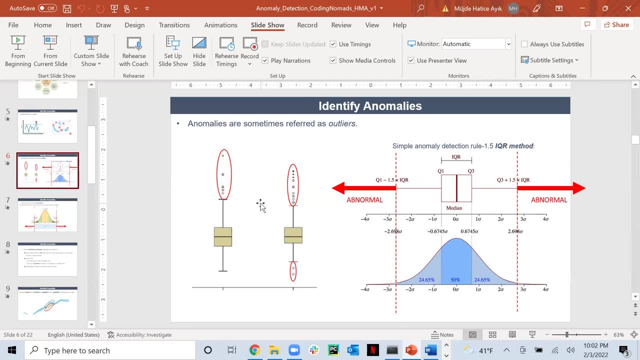 How are you doing the data preprocessing? In my case, when I mentioned about data preprocessing, Basically it's not only noise. I mean get filtering noise, It's some part of it. But when it is about filtering noise like, for example, this was a big problem for me when I was working for defense. 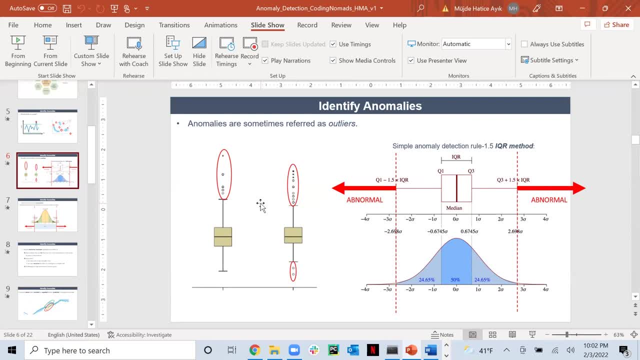 We had like sensory information and it was too noisy. Then I was coming together really with field experts, with avionics people, and say, OK, we need to filter this. But then they were telling me we should use this. There was a filter type but you couldn't use low pass filter. 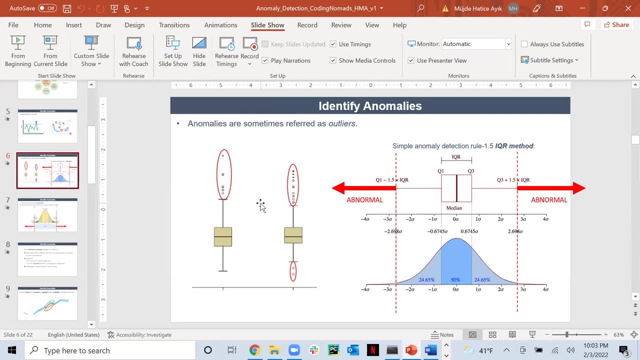 You couldn't use that filter but you could use. they said to me: like no lag filter, So you should filter it out smoothly, But you should. that filtering should not produce any lag in the response, any shift in the response. 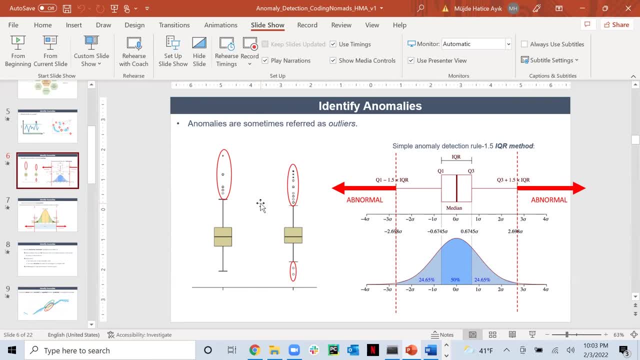 So those kind of things in terms of filtering was something really I was deciding together with field experts because physically, they know much better than I do In terms of, like, sensor information, Other things like, for example. I mean, to me really data processing is very important stage and we should always work with cross-functional teams, even in data preprocessing stage. 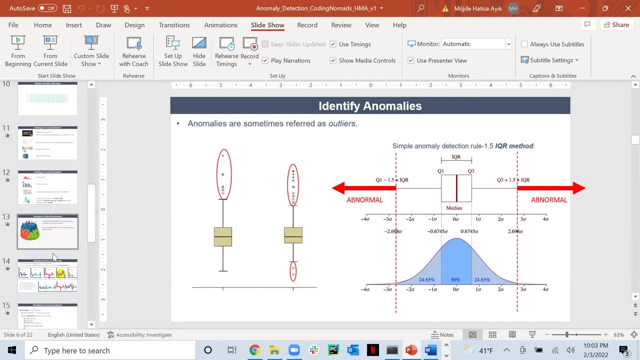 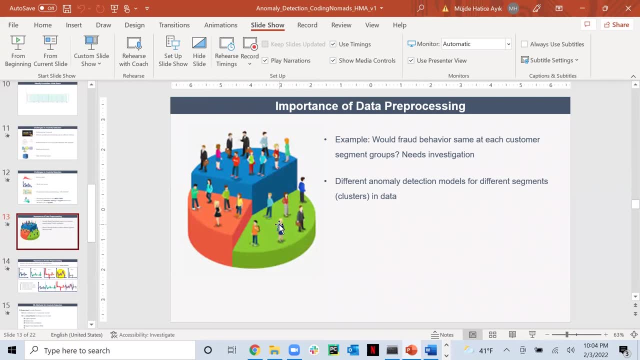 For example, when we have customer segments different like this, I mean I even go to them and ask beforehand: we think we should have different thought models for this, Because I mean, Yeah, They know the business very well. They may think that I think maybe you can first try the same model for all of them and see if it works. 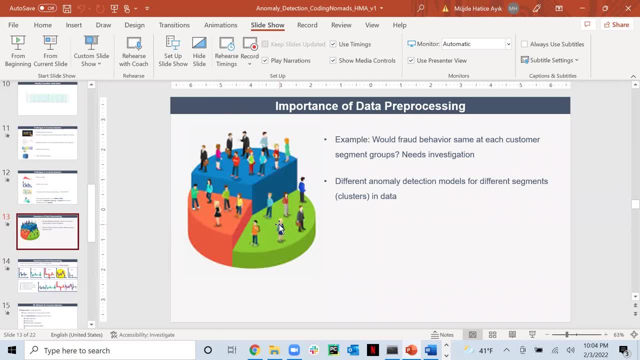 Or if you end up with like this doesn't work for each cluster, they would say, okay, that makes sense because they behave differently. So I mean coming together with them and just exchanging ideas is really important. Other things are basically dealing with features, outlier detection. 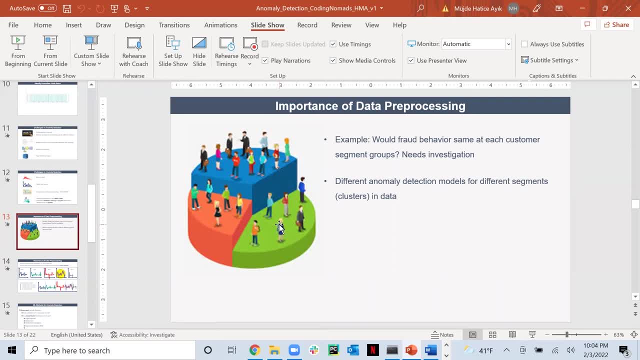 Missing value. I mean filling in missing values, Dimensionality reduction, All data science stuff. But other part is really about the business and field experts know that very well. Thank you, Yeah, Cool, So I think I've got to hop off. 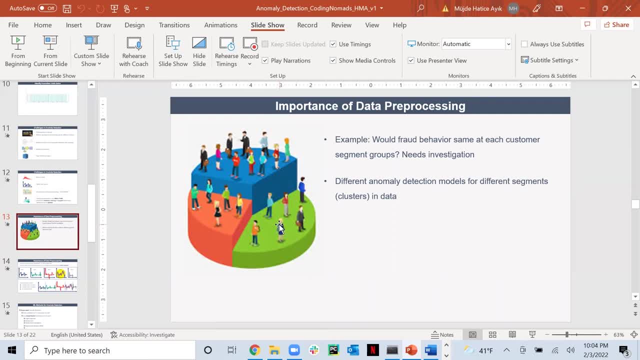 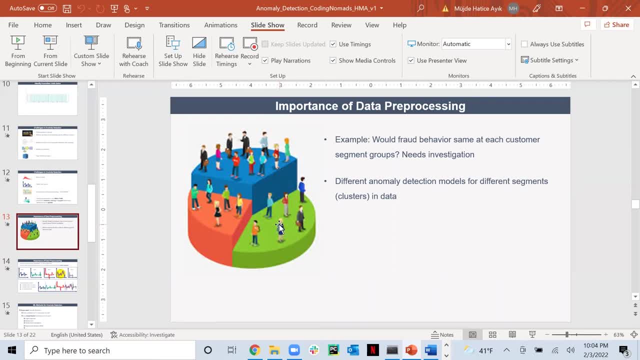 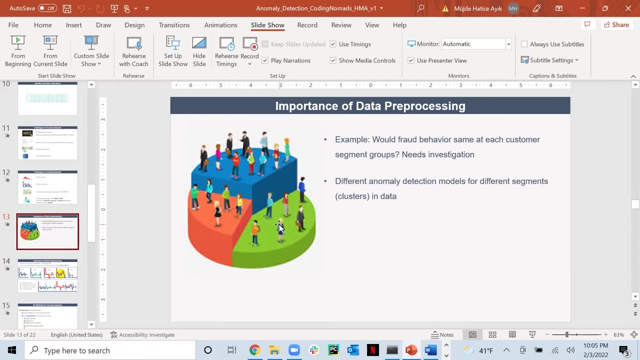 You're clearly, you've clearly spent a lot of time in this field and working with these tools and it's really neat to just listen to you talk And thank you also, Chadas, for joining And, as John said, just listen. 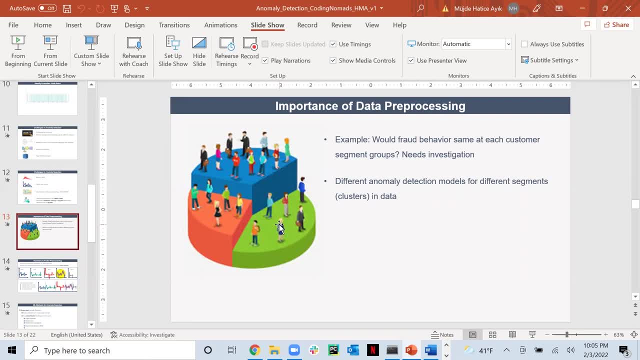 Yeah, Listening to the two of you go back and forth is is fascinating, So thank you for sharing that with us And- and I'll turn it back over to John, Yeah, Yeah, good to be in a room with a lot of smart people, especially a lot of people who are smarter about. 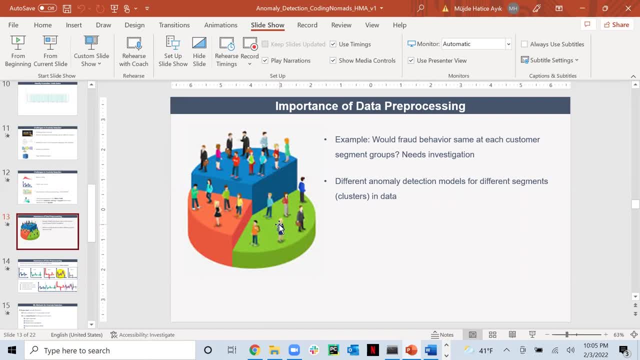 something than I am. It's a lot of fun, So this has been a great hour. Thank you, Mushta. I really appreciate you volunteering. Thank you for your patience and me getting back to you, And hopefully we're going to have you back again soon to talk about some more stuff with machine learning and. 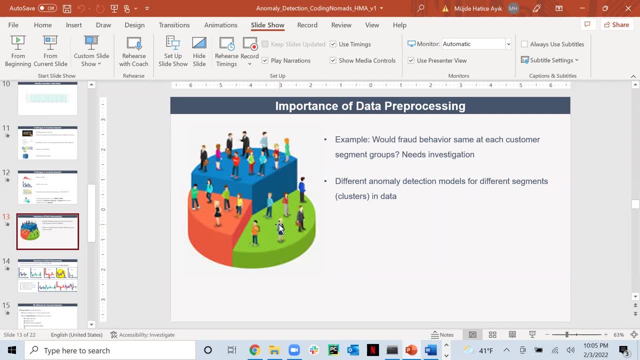 data filtering, data cleaning up, figuring out really cool ways to do this stuff. Um, our next tech talk is going to be in two weeks. Uh, Ryan, I believe you are up for that one. Uh, this one here is going to be on interviewing skills and how do you interview? 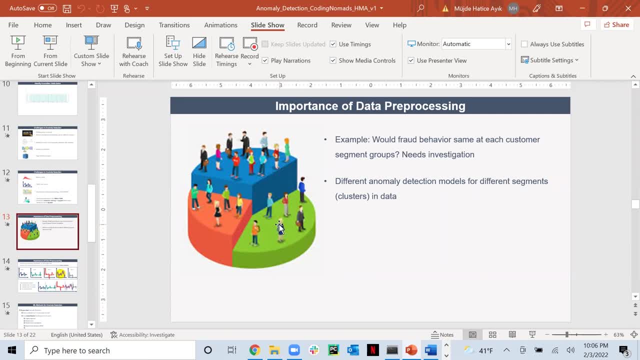 How do you get from where you are at Coding Nomads with all these cool skills and all this great knowledge and get yourself an actual job? So that's going to be a fun one as well. I'm looking forward to that. I'm looking forward to hear what other people have to think about interviewing. 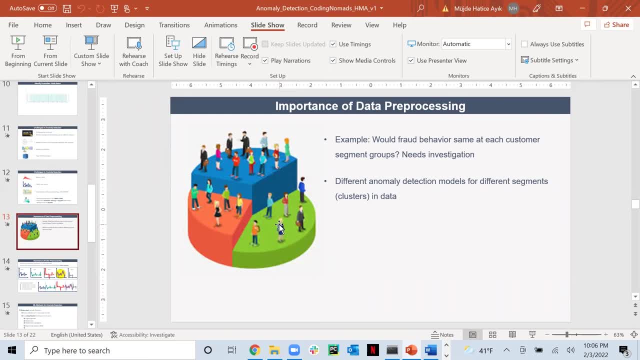 I've been on both sides of it and I'm really looking forward to that one Uh. we have another one uh right after that with uh Brandon Giygas, and he's going to be talking about Flask and building APIs. 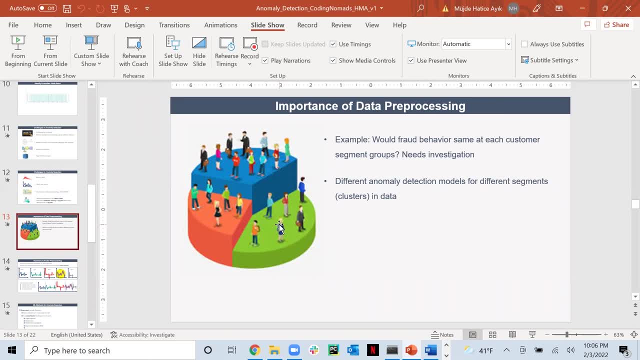 As well. Uh and then, uh, I don't have anything yet, but we're getting a couple of things lined up and we'll have some more exciting news about that here in the next coming week. So, uh, until then, stay safe. If you're stuck in this winter snow like I am, stay warm. Uh and uh, we will.